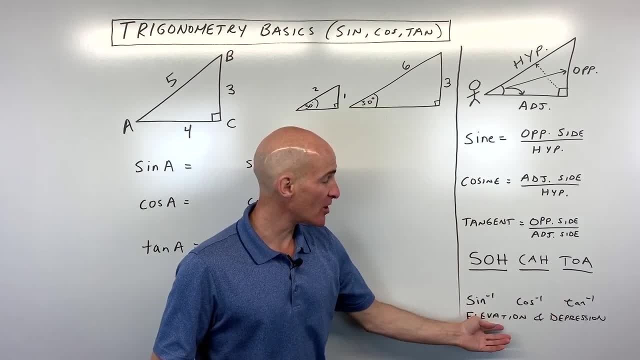 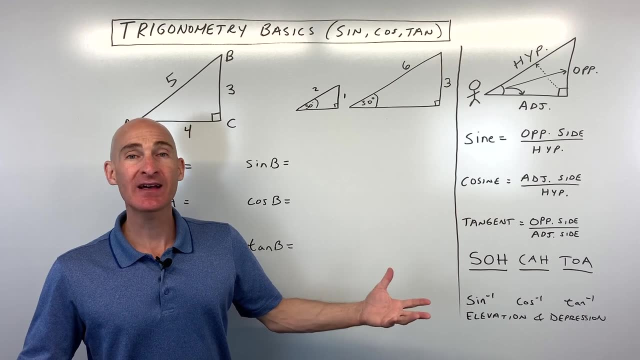 be doing the sine inverse, cosine inverse, tangent inverse, as well as talking about the angle of elevation and angle of depression. So let's dive right in. The first thing we want to talk about is you know what exactly is trigonometry? Well, if you look closely at the word, trig refers to. 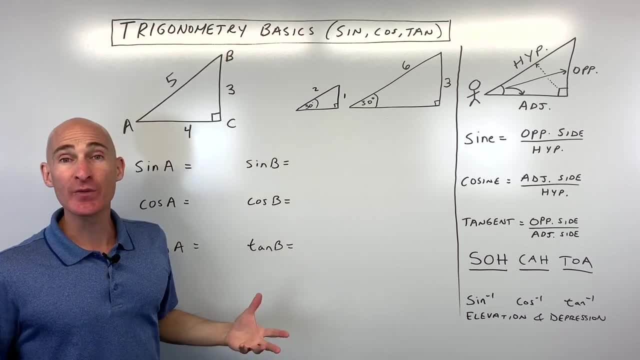 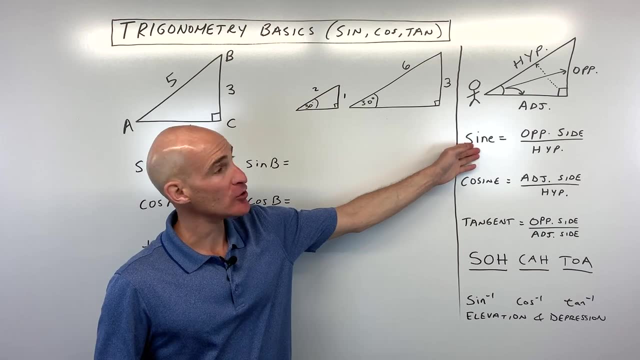 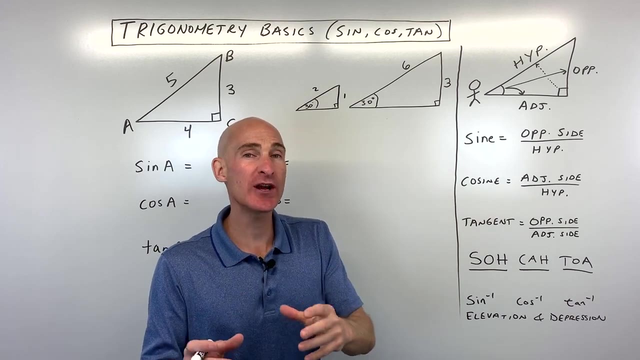 triangle, and metri refers to measurement, like the measurements in a triangle, whether it's the angles or the sides. So the first thing we want to talk about are the trig ratios, also referred to as the sine, cosine and tangent of an angle. Now, when we talk about a trig ratio, a ratio means 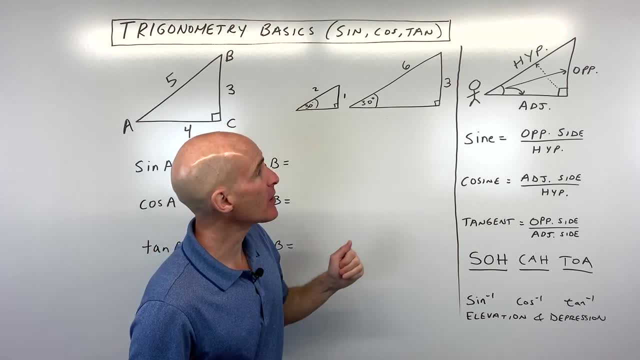 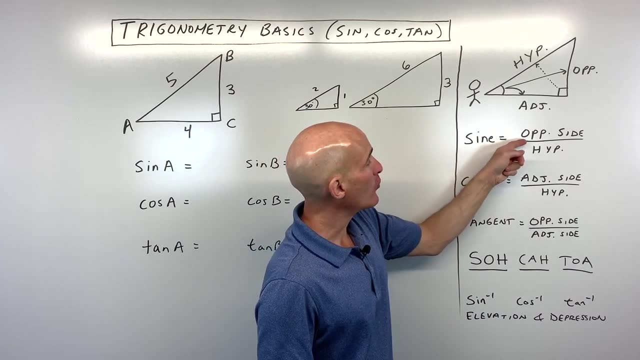 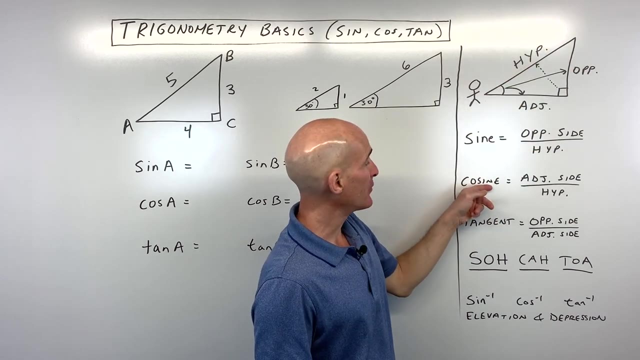 you're comparing two quantities And in this case we're comparing two of the side lengths in a triangle. So when we talk about the sine ratio, we're talking about the ratio of the opposite side length divided by the hypotenuse. If we're talking about the cosine, we're talking 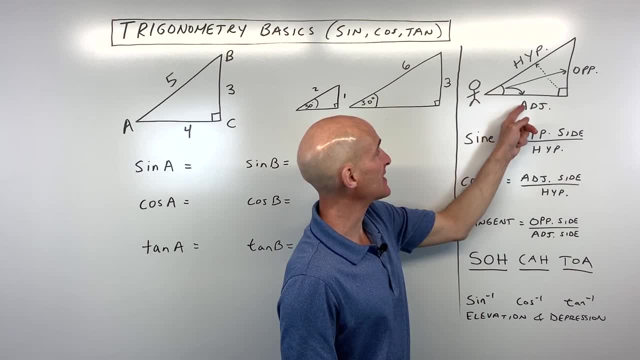 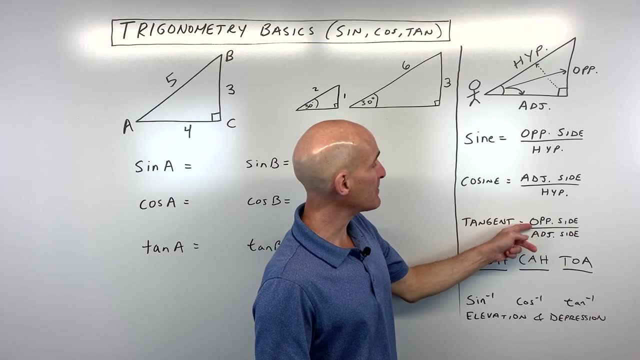 about the ratio of the adjacent side. okay, that's the side that's next to the angle divided by the hypotenuse, the one that's across from the right angle. And then the tangent ratio is the ratio of the opposite side, the one across from the angle divided by the adjacent side, the one next to the. 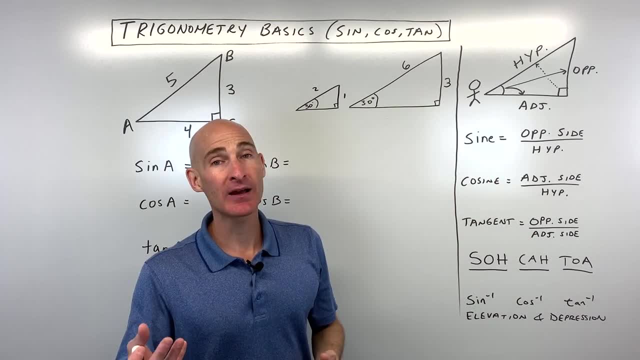 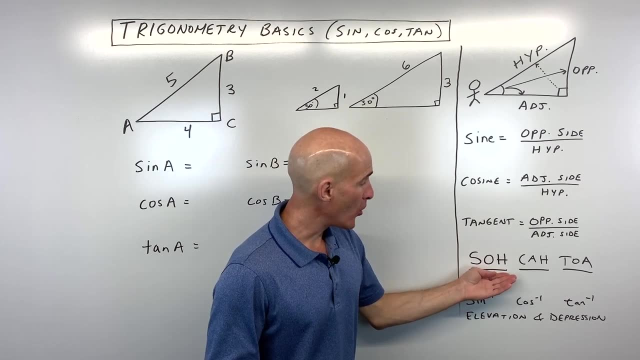 angle. Now you're probably saying, Mario, that's a lot to remember, And I completely agree with you, And that's why a lot of students, when they're learning trigonometry, the first thing they learn is this acronym: SOHCAHTOA. And what exactly? 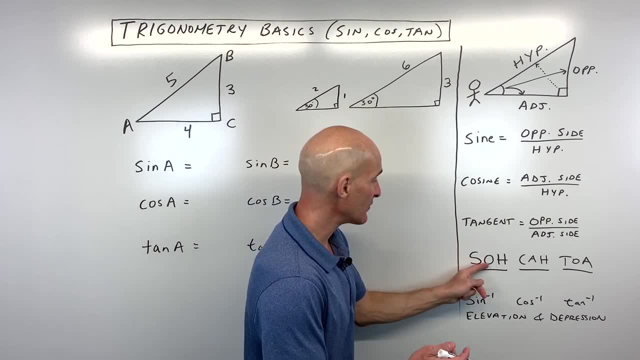 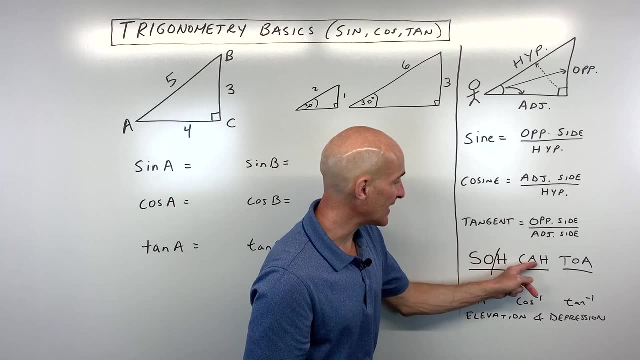 does that mean? Well, it means S, for sine is the ratio of the opposite side divided by the hypotenuse. The cosine is the adjacent side divided by the hypotenuse And the tangent is the opposite side divided by the adjacent side. 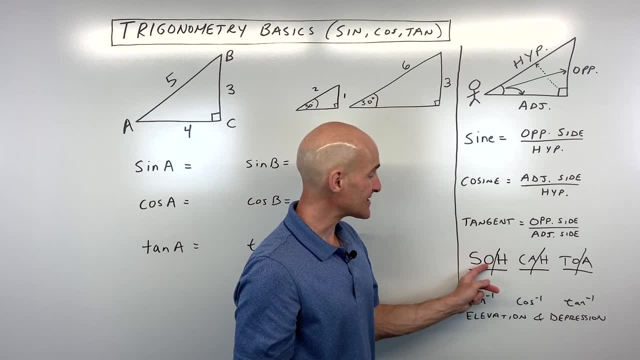 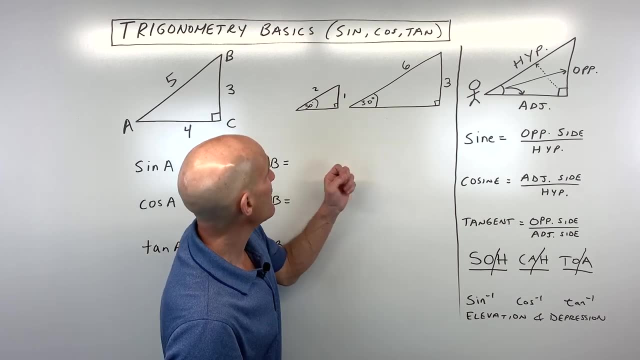 Remember SO-CA-TOA, and just remember it's the second letter divided by the third letter. You'll have those ratios. Now we're going to do examples with all these so you can get really good at it, And the first thing you want to understand, though, before I jump into an example, is: 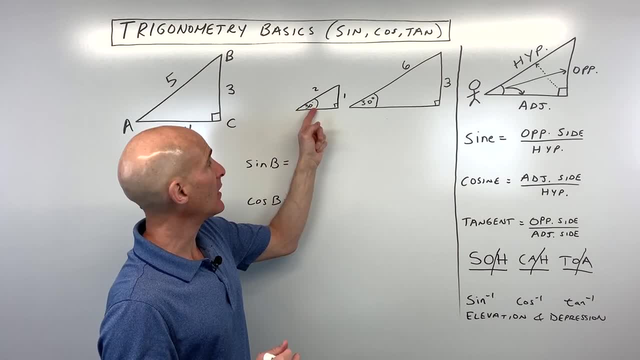 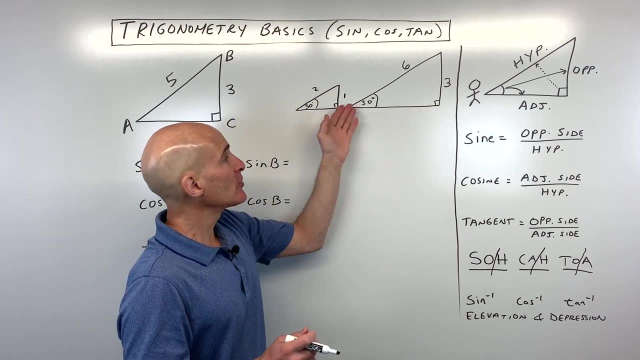 say, if you have a little triangle like this where it's a 30-degree angle and you've got a right angle, and here you have a larger triangle that has a 30-degree angle and this right angle, You probably learned in geometry that when you have two angles that are congruent to two angles, 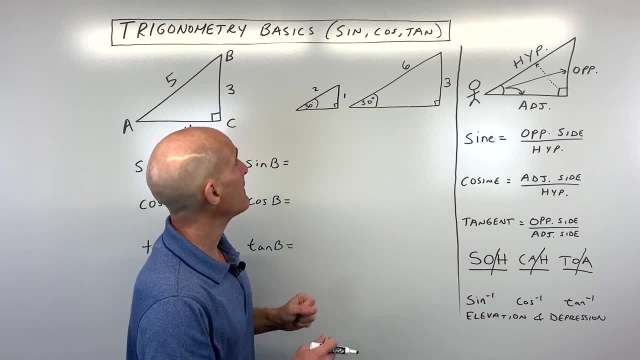 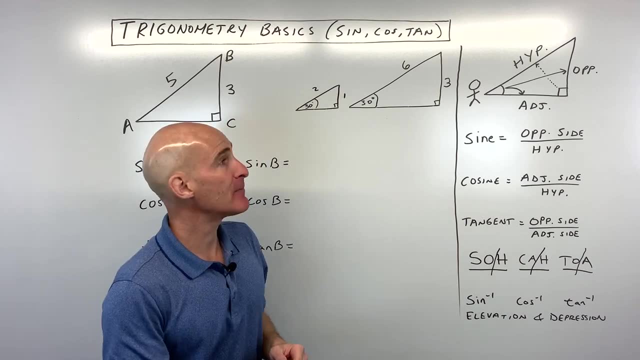 the triangles are what we call similar, And what it is is that one triangle is basically proportionally larger than the other triangle, or proportionally smaller, And what happens is that, if you're, let's say, we're looking at the sine of this angle, 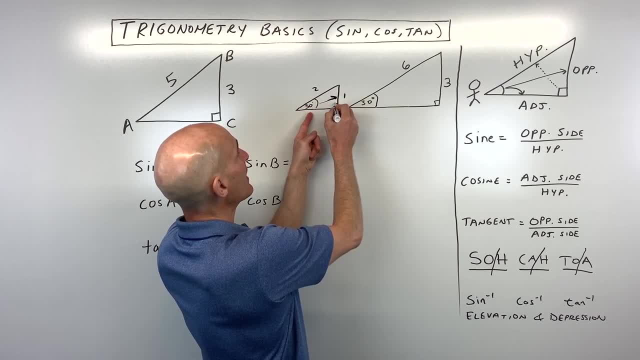 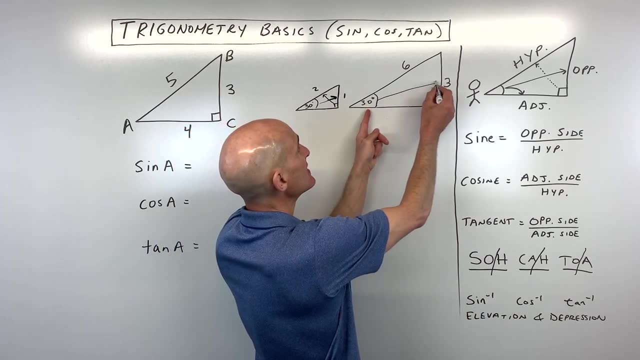 sine is the opposite side- okay, the one across- divided by the hypotenuse. See how that ratio is 1 over 2, 1 half, Whereas in this larger triangle here the sine of 30 degrees is the opposite side, 3, divided by the hypotenuse 6.. 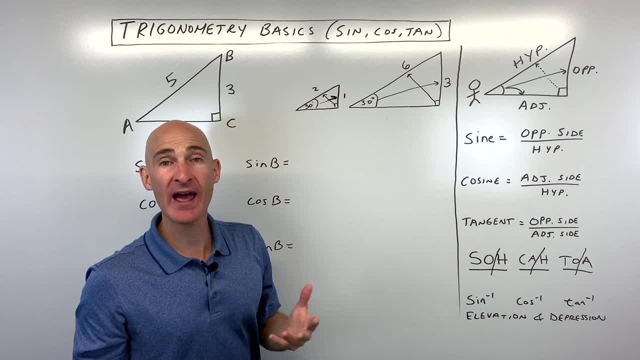 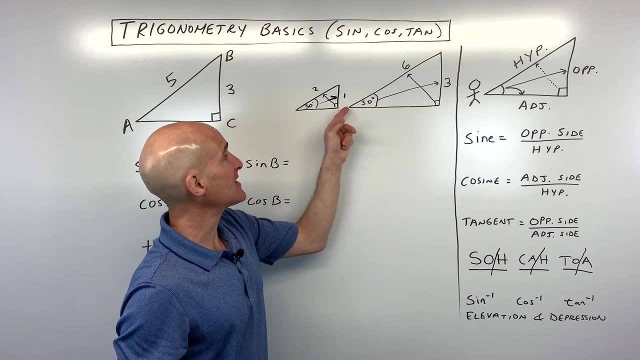 Well, 3 divided by 6 is the same as 1 divided by 2. That's 1 half or 0.5.. So that's really interesting when you're working with similar triangles or a right triangle that has that same acute angle. 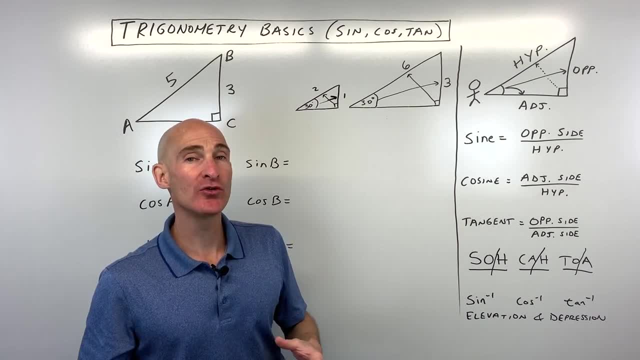 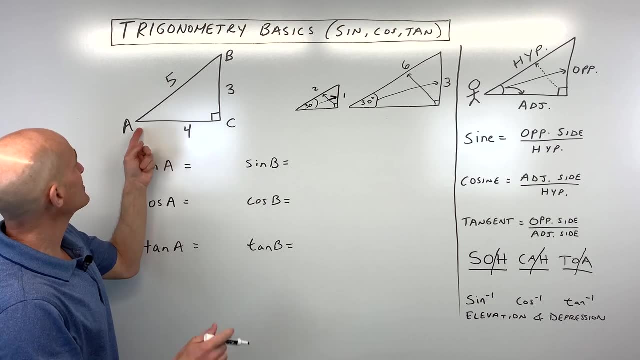 The corresponding sides are going to be proportional, so those trig ratios are going to be the same. So that's the real magic of trigonometry. But let's get into this first example, this introductory example. Say, for example: we want to find out the sine of angle A, the cosine of angle A and the tangent of angle A. 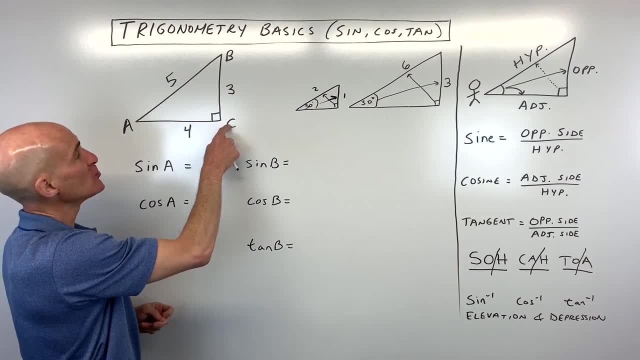 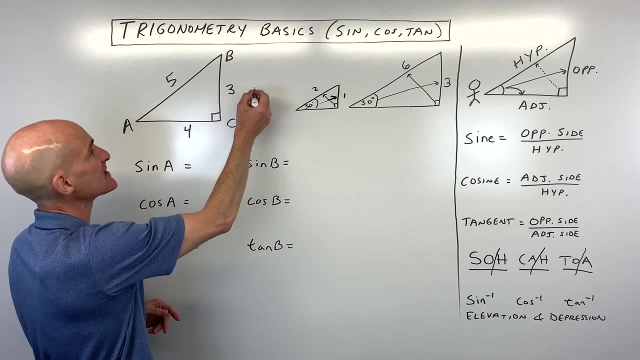 And one thing to notice is that when we talk about angles, we use capital letters, whereas when we talk about the sides across from the angles, we usually use a lowercase letter. So this would be like side A, like a lowercase a. So what exactly is the sine of angle A? 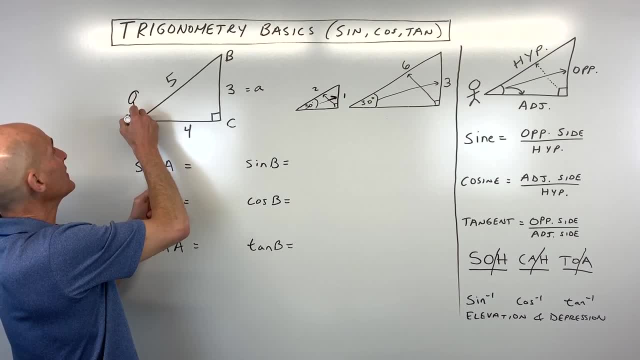 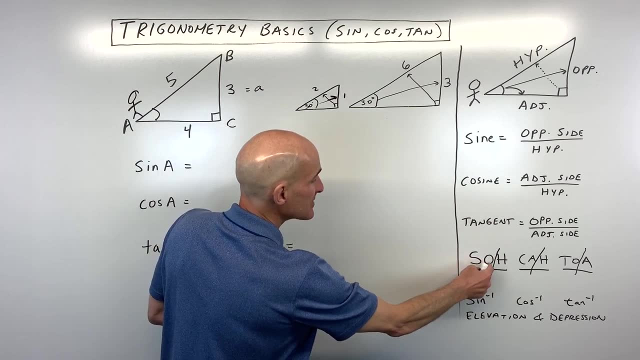 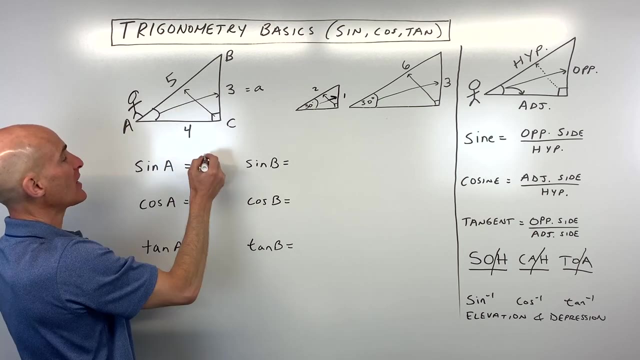 Well, the way I like to explain this is pretend like you're standing at that particular angle that you're working with. That's your perspective. So if you say, hmm, sine is the opposite divided by the hypotenuse. So opposite means across, that's 3, divided by the hypotenuse, that's the one across from the right angle. 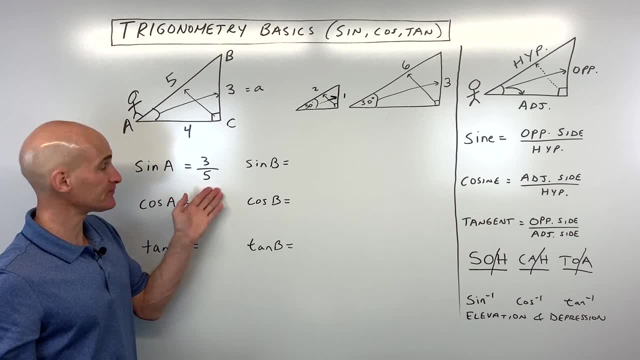 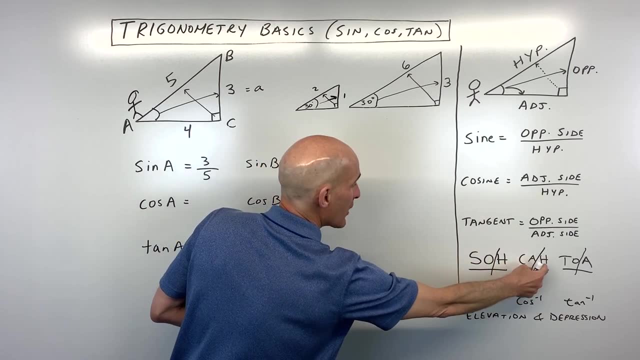 That's 5, so the sine of angle A is 3 fifths. How about the cosine of angle A? Well, cosine, we know, is cosine, is adjacent over hypotenuse, see the ka. So adjacent means next to, that's going to be 4,. 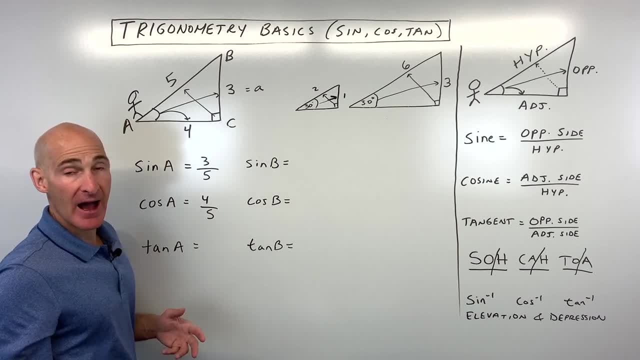 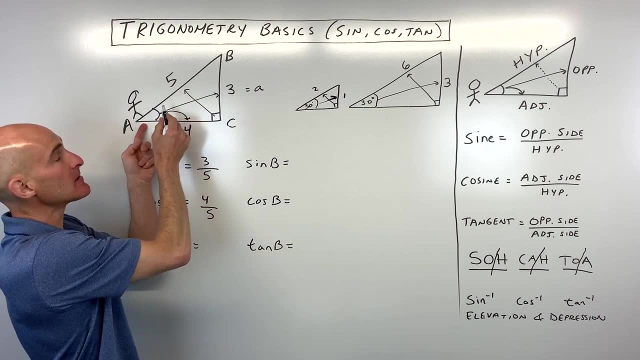 divided by the hypotenuse which is across from the right angle, 5.. Now some students go a little bit off the track here where they'll say, well, adjacent isn't that? this one here isn't 5 adjacent. 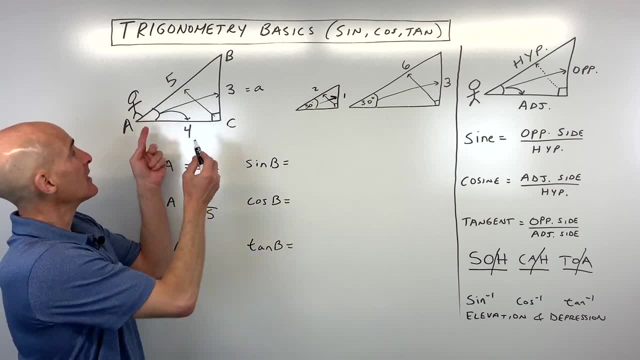 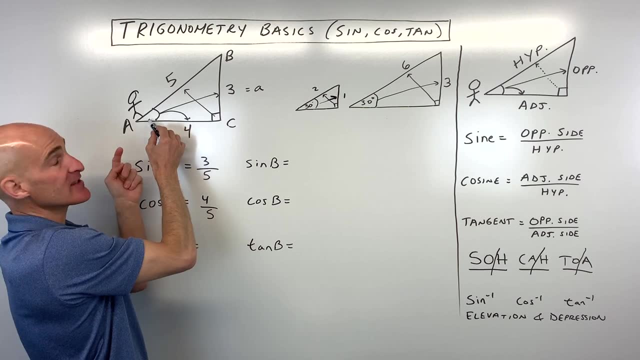 Adjacent in everyday language means next to right, But this one, the 5, is always going to be the hypotenuse. it's always the one across from the right angle. So adjacent is going to be the other side, that's next to this angle A. 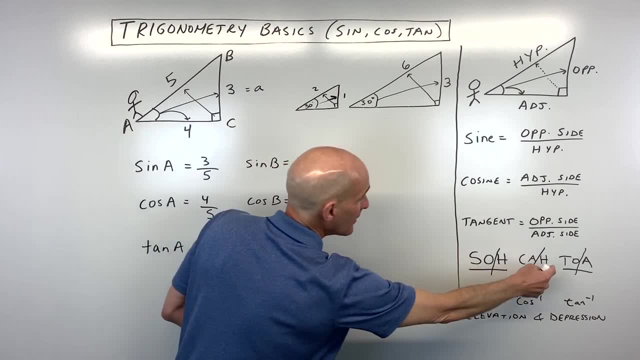 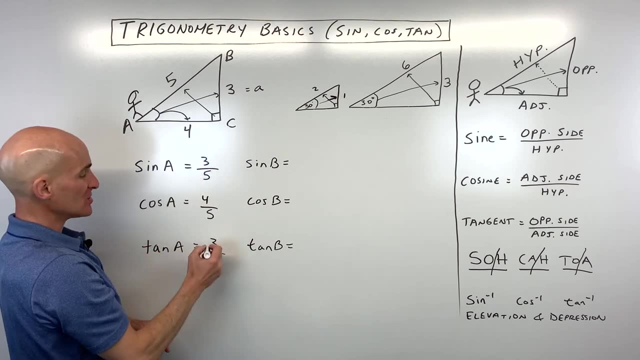 Now, with tangent of angle A, we're doing TOA. so that's opposite over adjacent. That's going to be opposite, which is 3, divided by adjacent, which is 4.. Now, another thing that students sometimes like to do is as soon as they get the triangle and they're working with angle A. 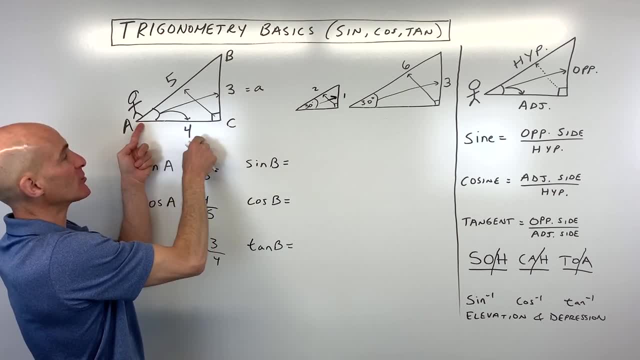 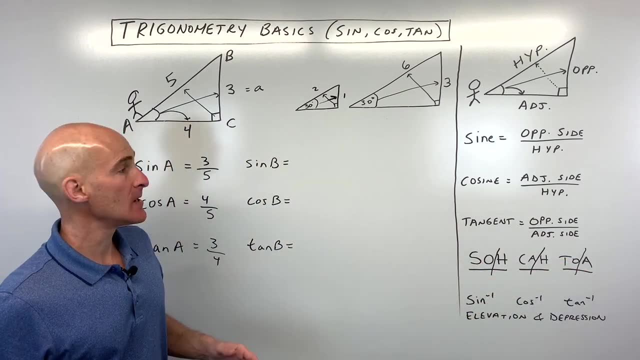 they'll just label opposite and they'll write opposite here adjacent. they'll write adjacent here: Hypotenuse, hypotenuse. And then they can just use their SOHCAHTOA- you know acronym- to help them with those ratios. 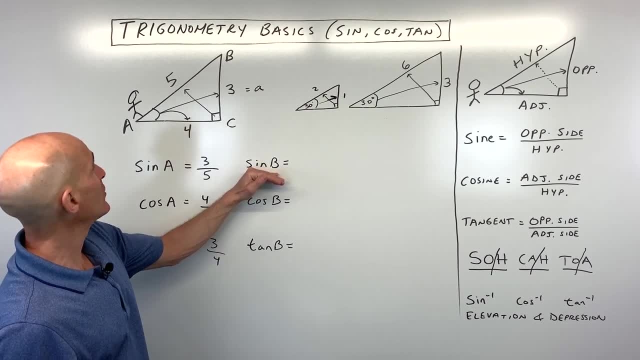 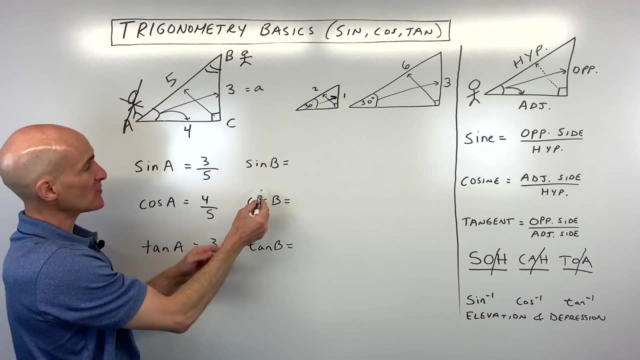 Let's switch over to sine of angle B now. So here what we're doing is we're no longer over here, okay, We're standing at angle B, we're at this angle and that's our perspective. So we say: what's the sine of angle B? 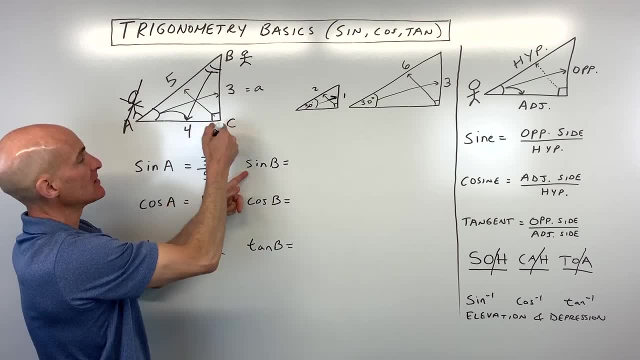 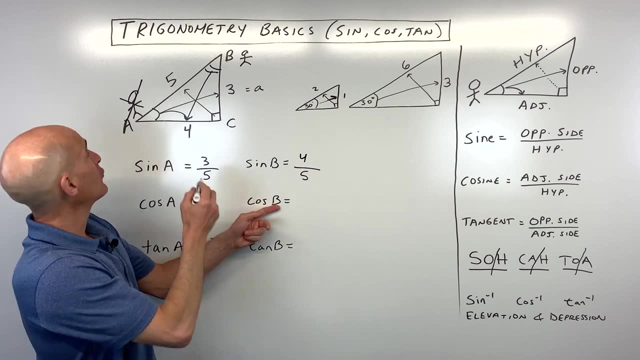 Well, that's going to be opposite. okay, the one that's across, that's 4, divided by the hypotenuse, that's one that's across from the right angle 5.. How about the cosine of angle B? 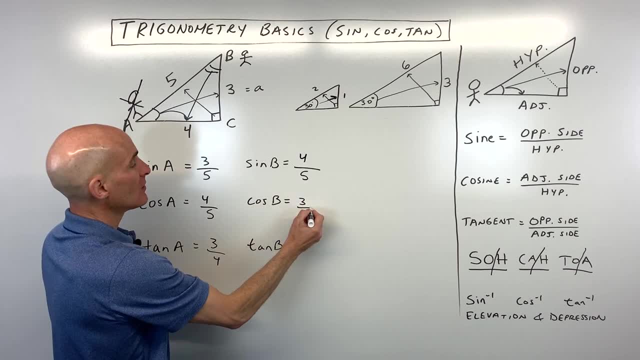 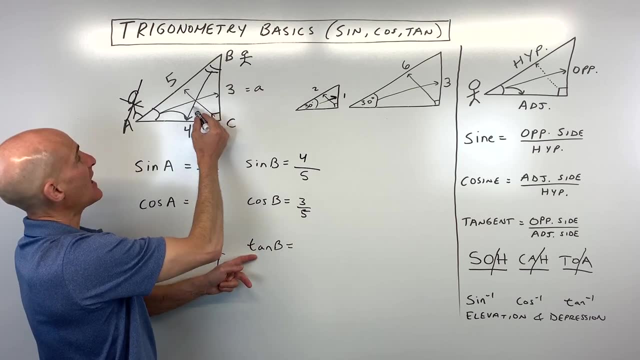 Well, cosine is adjacent, that's 3, over the hypotenuse, that's across from the right angle 5.. And what about the tangent of angle B? So, tangent is opposite, that's 4, over adjacent, that's the one next to here, which is 3.. 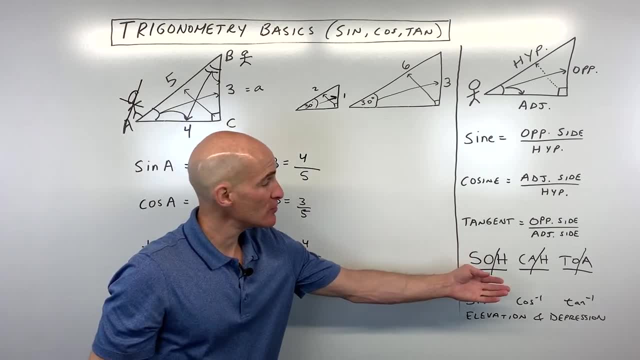 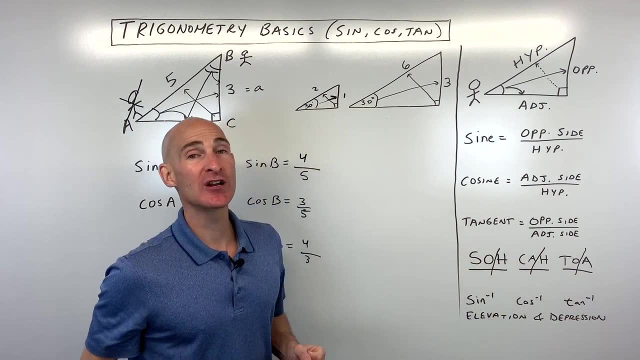 Again, we don't want to use the 5, that's the hypotenuse. So again, if you can just remember SOHCAHTOA and just remember it's always the second divided by the third, you'll have those trigonometric ratios. 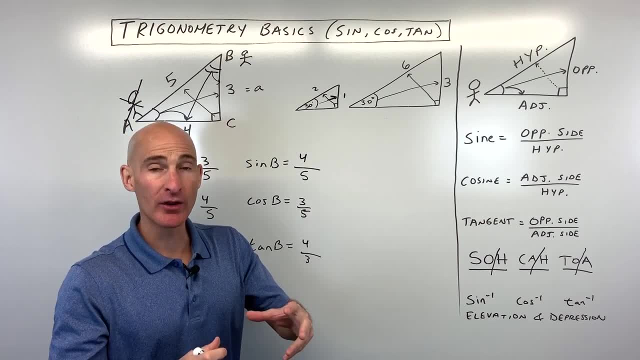 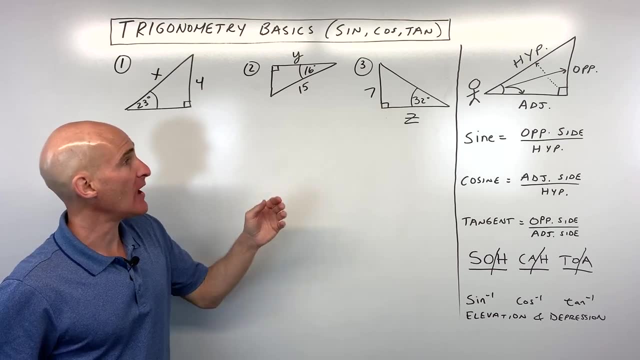 So now let's get into some other example problems where you're given the angle and you want to find the missing side. So everything that we've been working on in this lesson so far, this is right: triangle trigonometry, meaning that you have a triangle with a 90 degree angle. 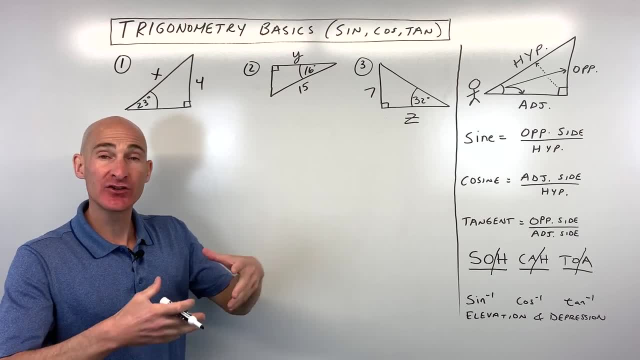 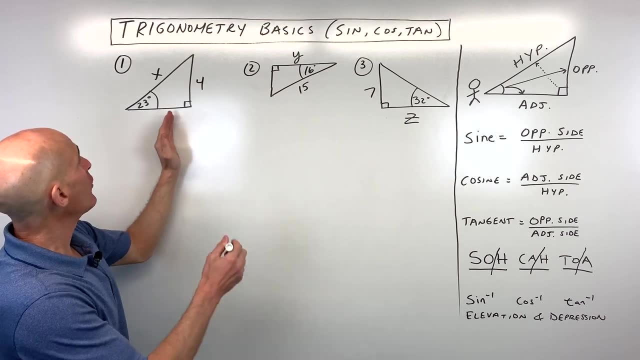 There's other problems that you can do not, involving a right triangle, where we get into the law of sines, the law of cosines, which is different from just our regular sine and cosine. For number one, though, we want to solve for this missing side here, this x okay. 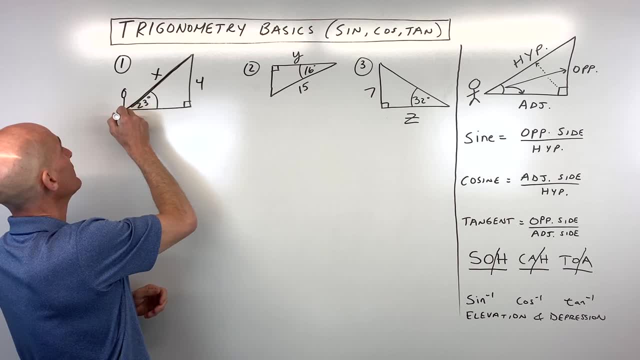 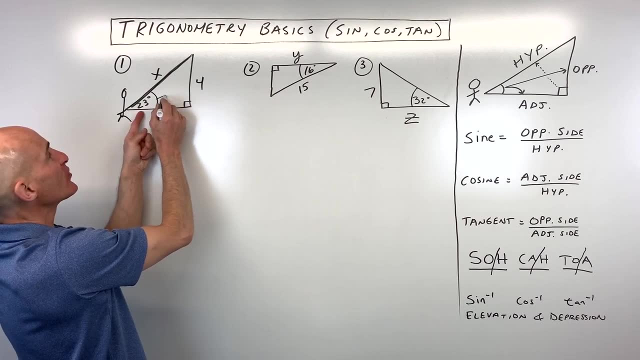 So what you want to do is you want to position yourself at the angle right, And then you say: well, what trig ratio sine cosine or tangent ties together this 23 degree angle, this opposite side 4, and this hypotenuse x? 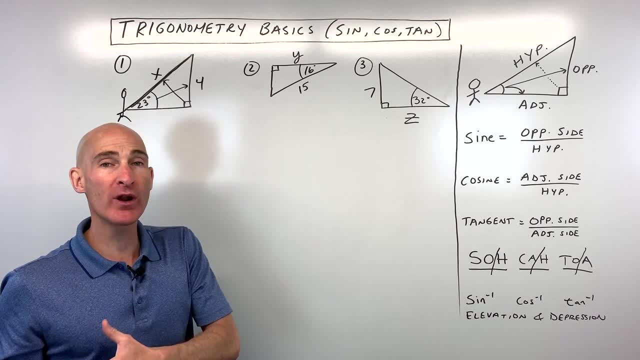 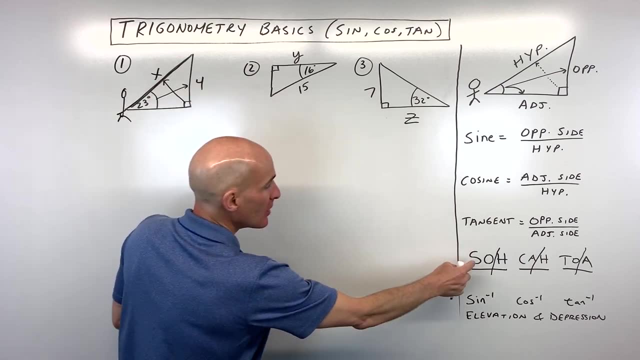 And you only want to have one unknown, one variable. If you have more than one unknown, more than one variable, you're not going to be able to solve it. So in this case we have- let's see opposite and hypotenuse. 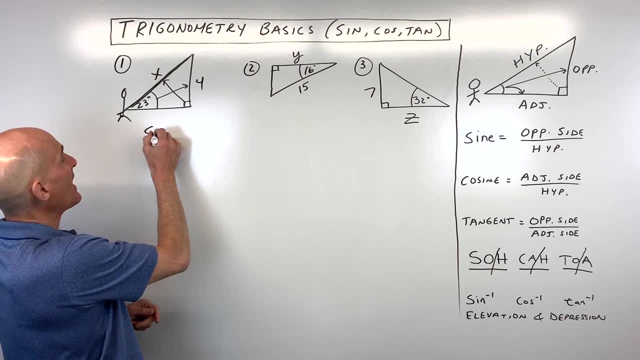 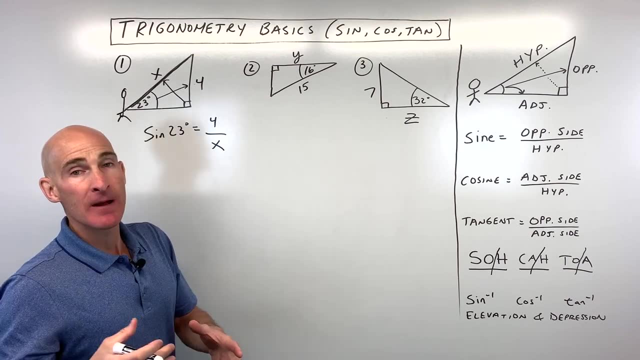 Oh, opposite and hypotenuse, that's sine. So we say: the sine of 23 degrees equals the opposite side, which is 4, divided by the hypotenuse x. Now what you can do is you can think of this as sine of 23 divided by 1,. 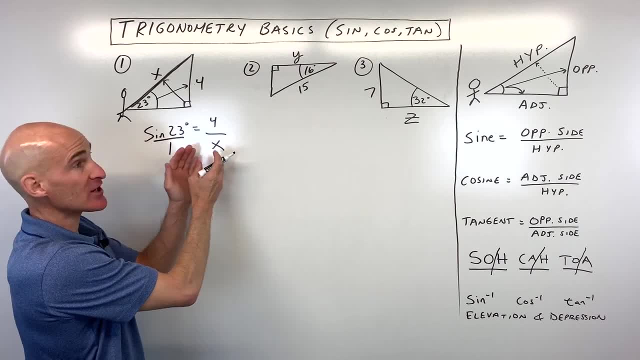 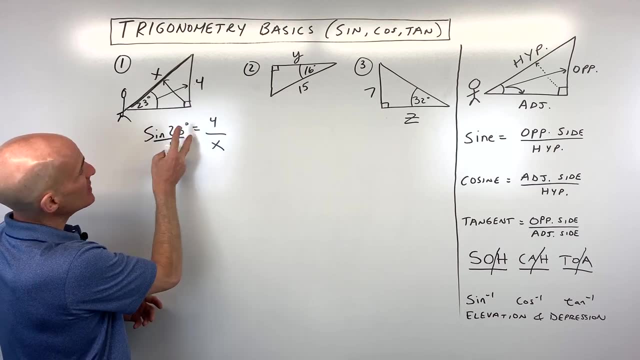 and now what we have is a ratio equal to a ratio or a fraction equal to a fraction. This forms a proportion, and we can use the properties of proportions to solve. So one way to do this is you can interchange these on the diagonal. 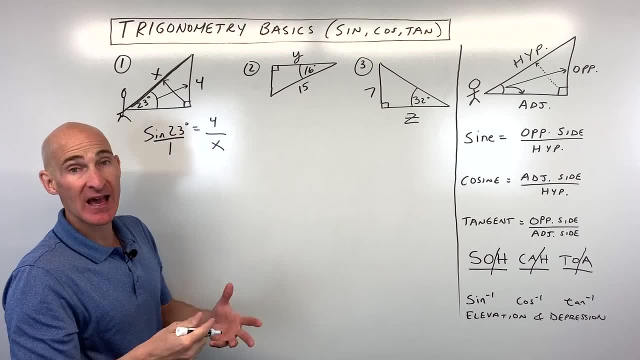 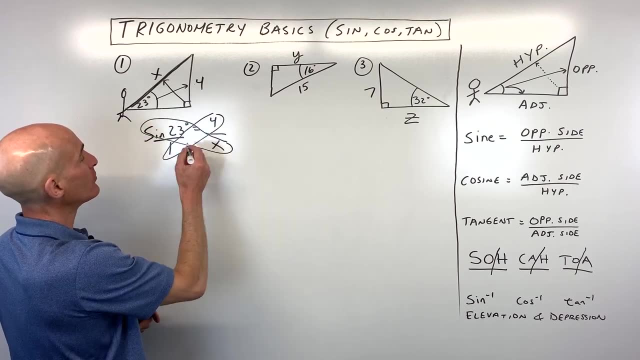 I could put x here and sine of 23 here. x divided by 1 is just x and we've got the variable by itself. But what I find is a lot of students, they just like to use that cross product property. They like to just cross multiply. 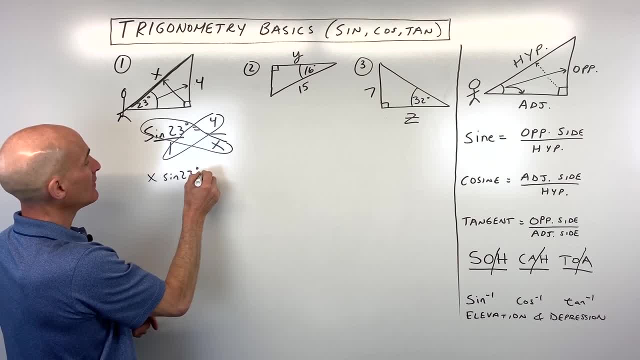 So x times the sine of 23 equals 4 times 1, which is 4.. Then to get x by itself, we're just going to divide both sides by the sine of 23 to keep the equation balanced, And we have x by itself. 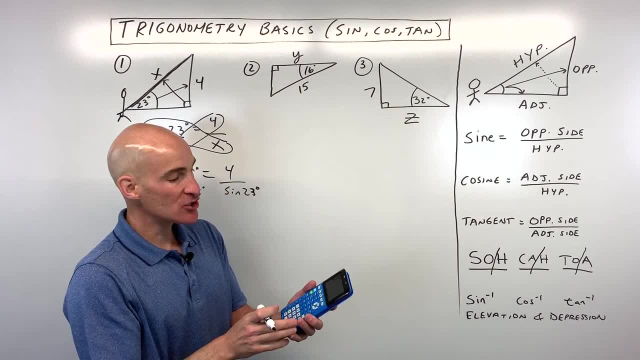 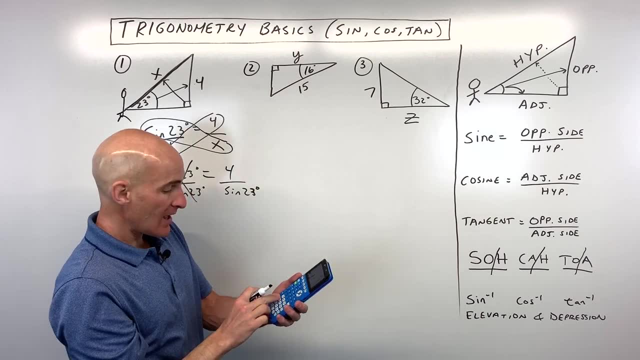 So now we're going to go to the calculator And when you do these problems you want to make sure you go to your mode and make sure that you're in degrees, because you can see, this angle is in degrees. So now we're going to go: 4 divided by the sine of 23 degrees, which comes out: 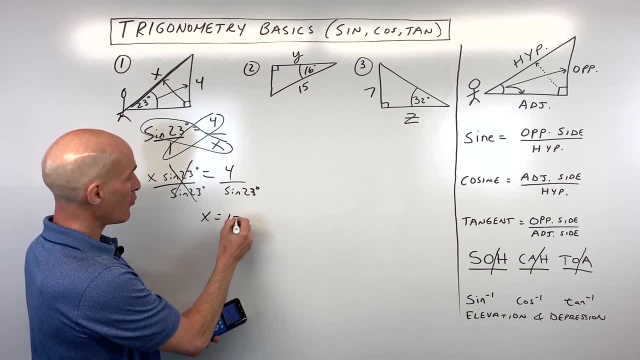 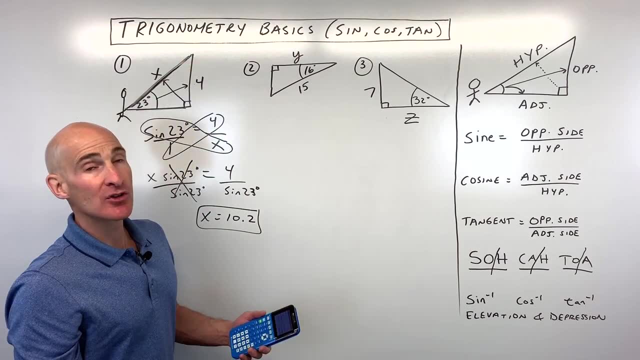 to. I'm just going to round to the tenths. This is about 10.2, and that's the length of this side, right here the hypotenuse. And you got it. So let's go to another example. see if you can do this one number 2.. 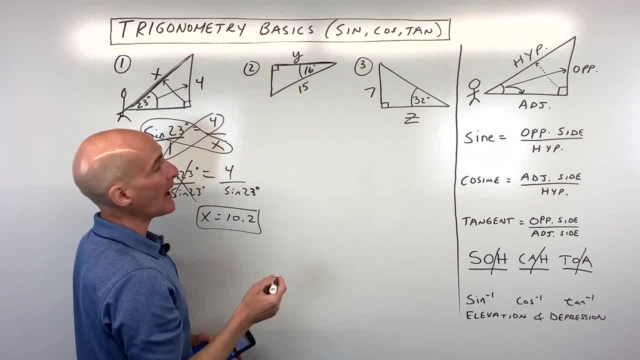 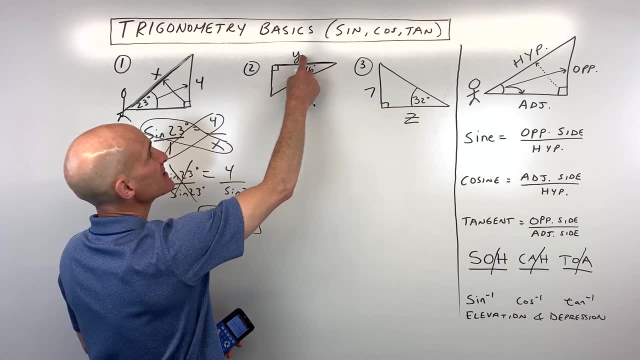 So, number 2, we're trying to solve for this missing side here, y. But we have to ask ourselves what trig ratio, sine cosine or tangent, ties together this angle, this side and this side. Well, again, remember, you want to position yourself at the angle. 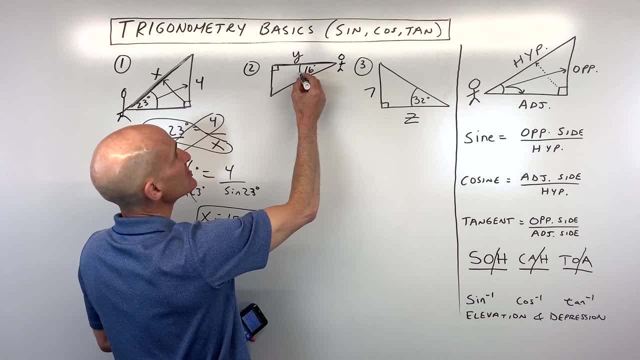 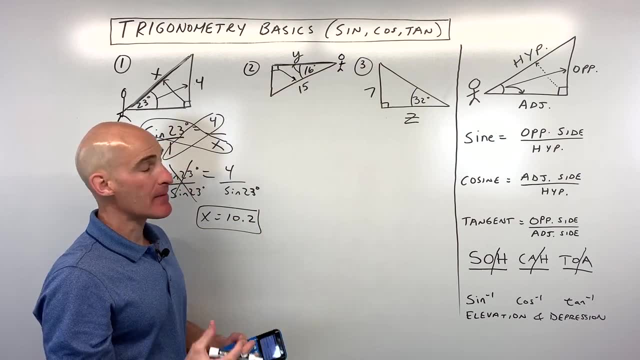 You want to pretend like you're standing at the 16 degree angle And then you say this is the adjacent side, because you're next to This one across from the right angle is the hypotenuse So adjacent and hypotenuse? OK, that looks like ka, which is cosine. 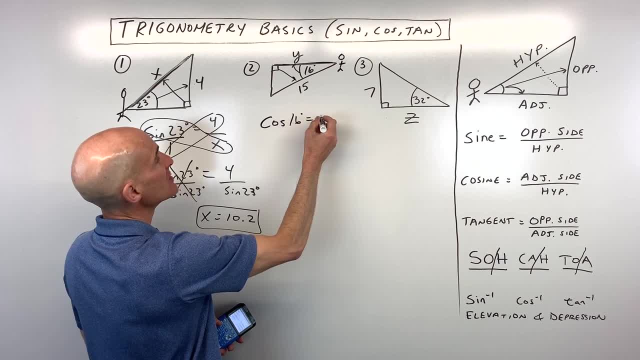 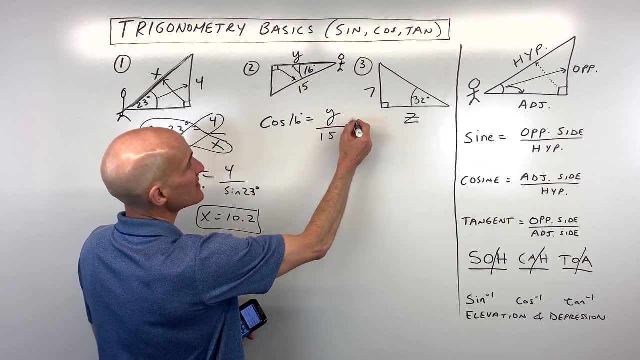 So we're going to say the cosine of the angle, cosine of 16 degrees, equals the adjacent side divided by the hypotenuse. Now all we have to do to solve is we want to get y by itself. So instead of dividing by 15, we're just going to multiply both sides by 15.. 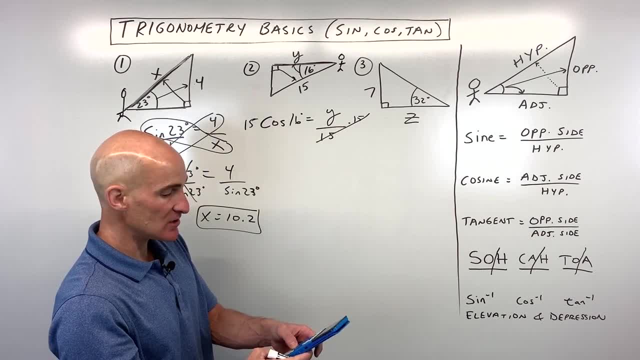 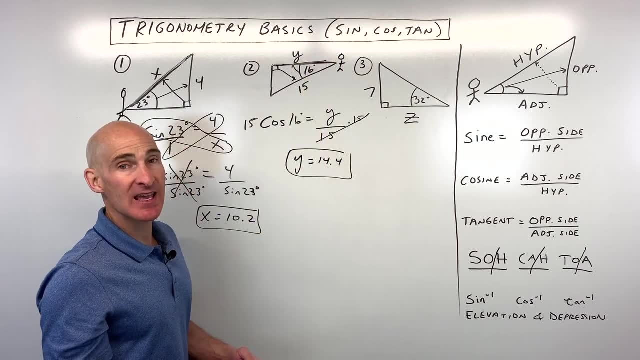 So we have 15 times the cosine, cosine of 16 degrees, which comes out to 14.4.. And you've got that missing side. One last example: working with these side lengths, what trig function do you think ties together this angle, this side and this side? 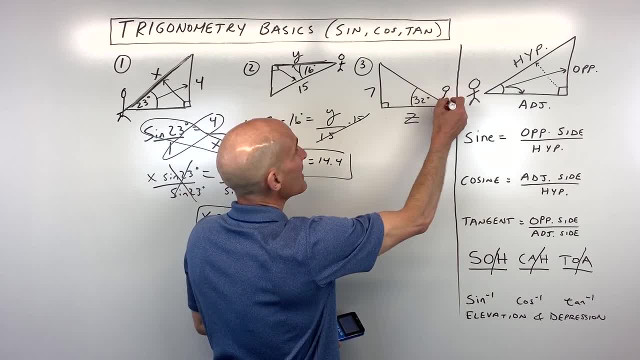 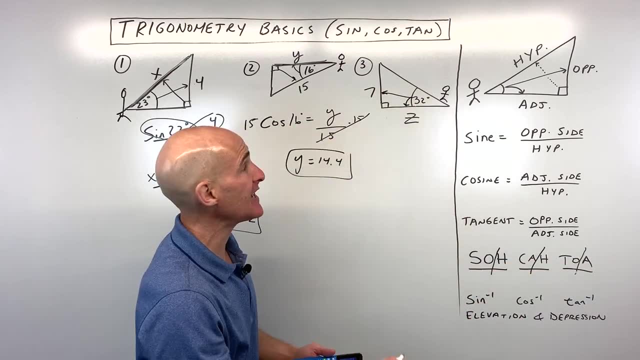 Is it sine cosine or tangent? Well, again, let's position ourselves at the angle. We've got opposite and adjacent. So, oh OK, opposite, adjacent, That's TOA. so this is the tangent. So we have the tangent of 32 degrees. 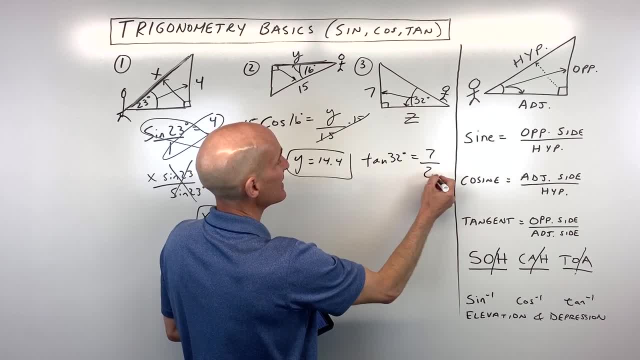 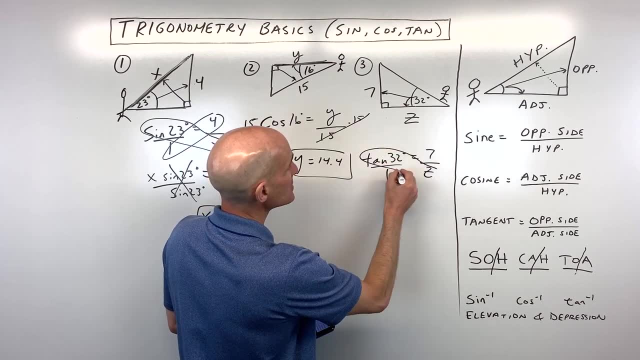 which equals the opposite side 7, divided by the adjacent side z. And then again we can use that property of proportions where you can switch these on the diagonal, or we can just do the cross product property. We'll just cross multiply. 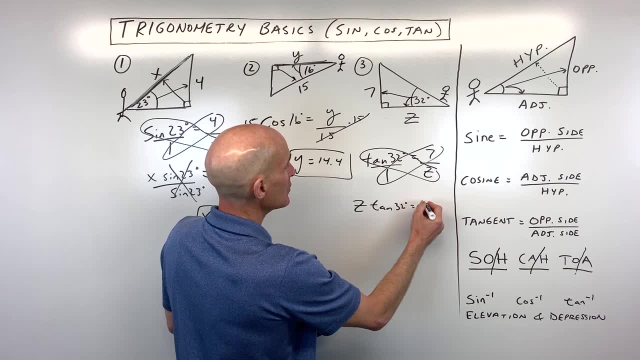 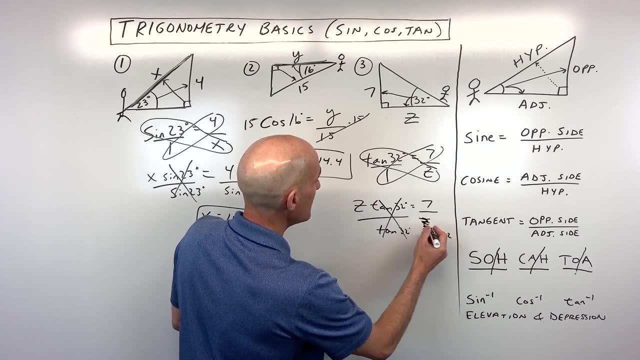 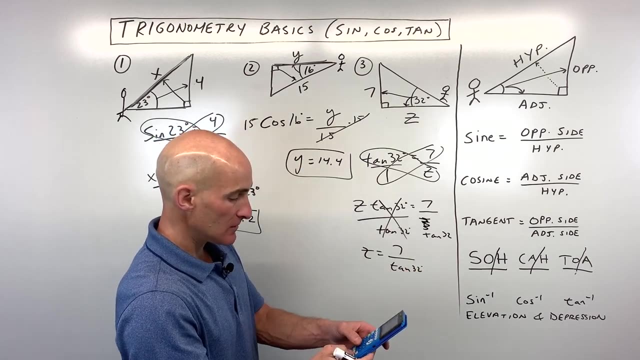 So z times the tangent of 32 degrees equals. So now we're just going to divide by the tangent of 32, to both sides of the equation, And now we have z equals 7 divided by the tangent of 32 degrees, which comes out to 11.2.. 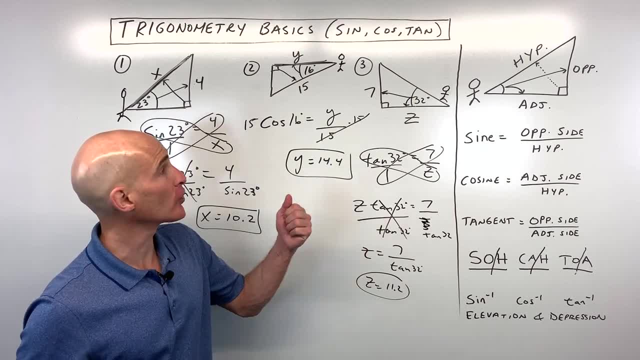 And you found the missing side. So the next thing we want to do is we want to talk about how do you solve for when you don't know the angle, but you know the side lengths, And that's where the sine inverse, cosine inverse. 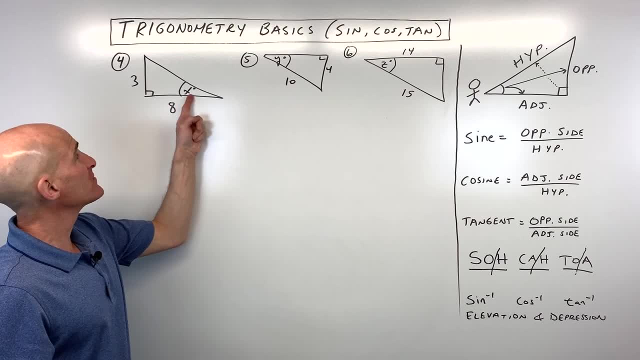 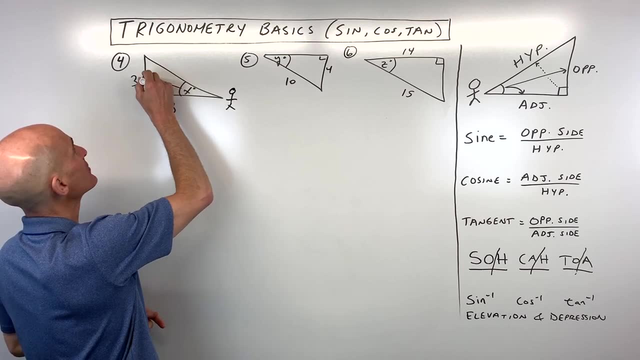 and tangent inverse come into play. OK, number four, we're looking for this missing angle x. So what we want to do is same idea. You want to position yourself at the angle and you say what trig ratio ties together the opposite side. 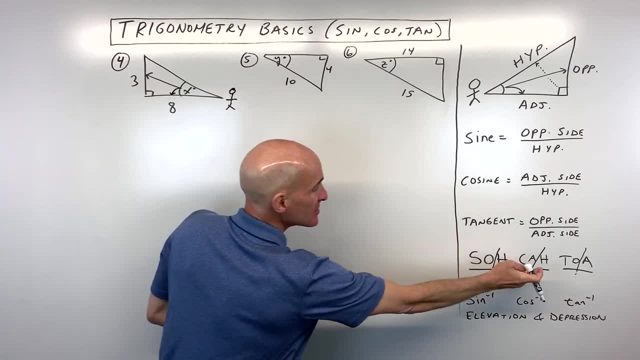 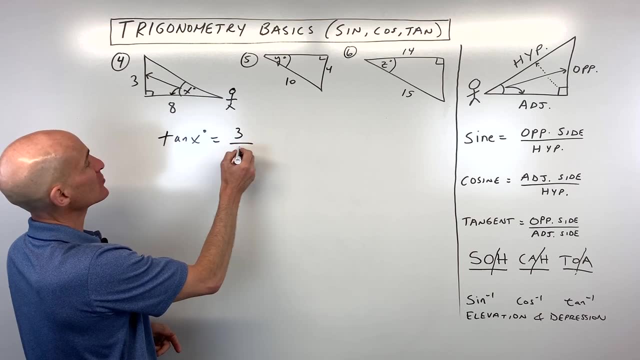 and the adjacent side. So we're going to take the tangent from this angle. Well, opposite and adjacent. we know that's TOA. So we're going to say the tangent of x degrees equals the opposite side, which is 3,. 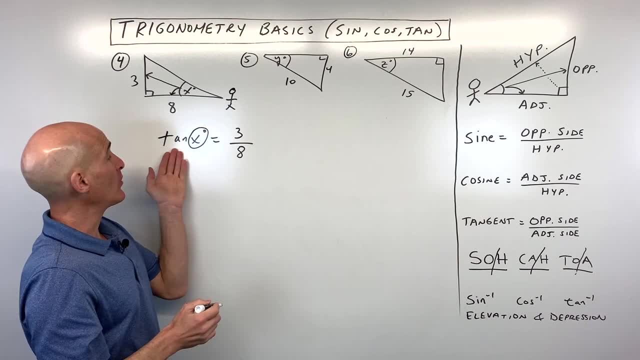 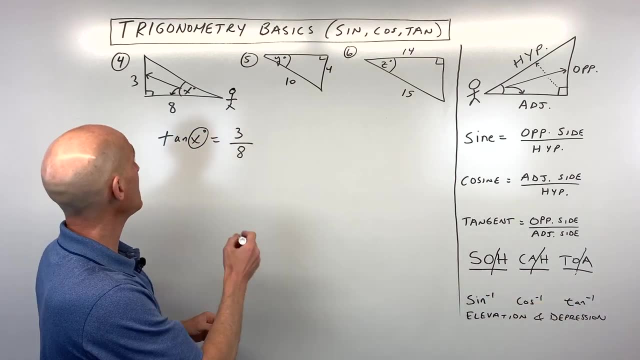 divided by the adjacent side, which is 8.. Now the thing is, we want to get this angle by itself, But we have tangent of x. How do we get rid of this tangent? That's where the sine inverse, cosine inverse. 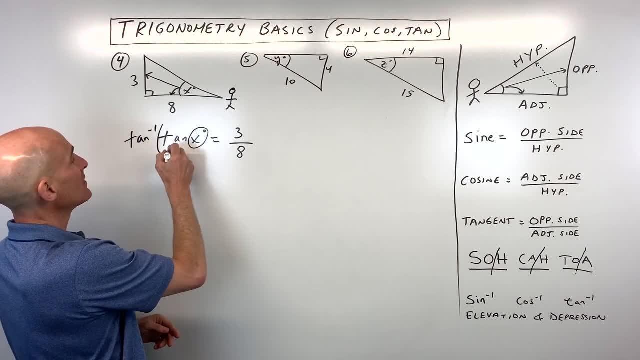 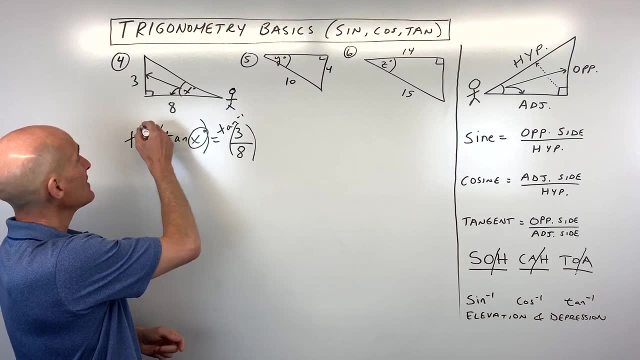 and tangent inverse come into play. So what we're going to do is we're going to take the tangent inverse of the left side. We're going to take the tangent inverse of the right side. Keep this balanced. These are inverses, They undo one another and we get the angle now by itself. 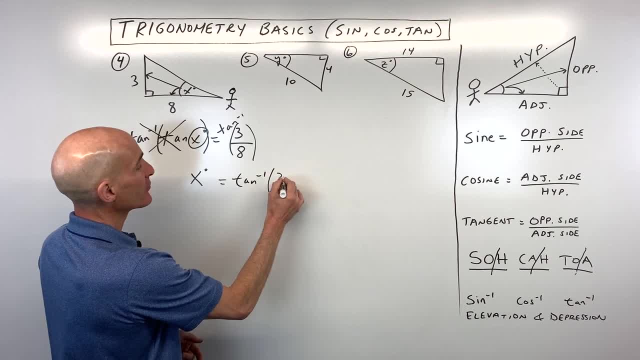 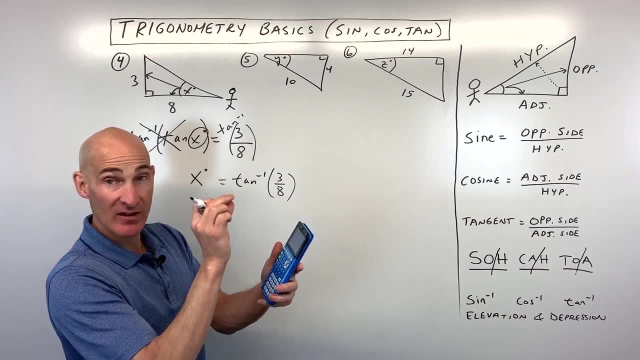 So x is equal to the tangent inverse of 3 over 8.. So we're going to go to the calculator again now And you'll probably notice, right above the sine cosine tangent you see the sine and you've got that minus 1,. 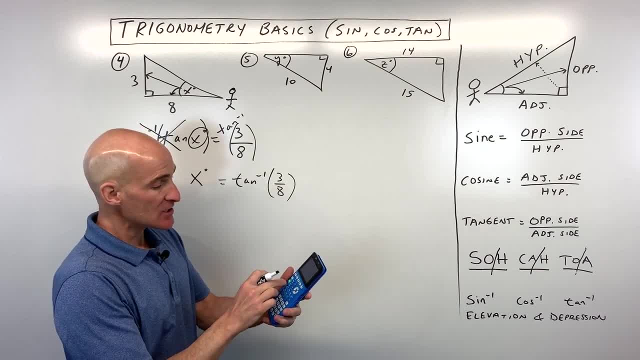 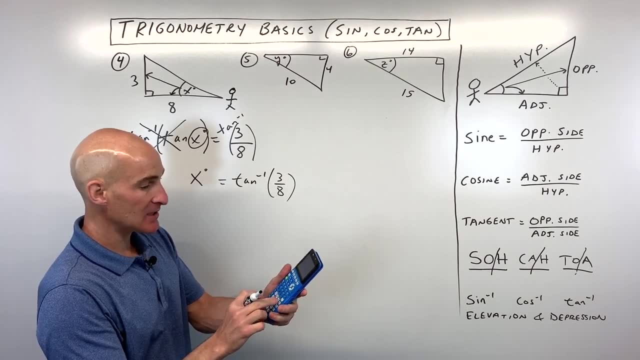 or cosine minus 1, or tangent minus 1.. That means the inverse. So you want to press that second key. I'm on a TI-84 here. So second tan inverse of 3 divided by 8. And that comes out to about: 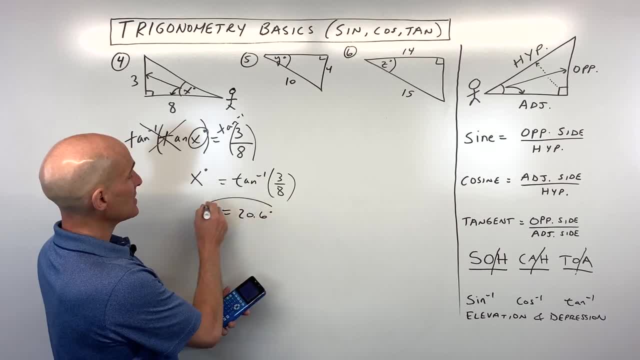 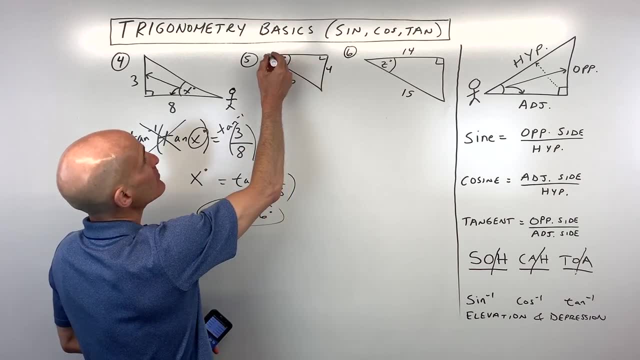 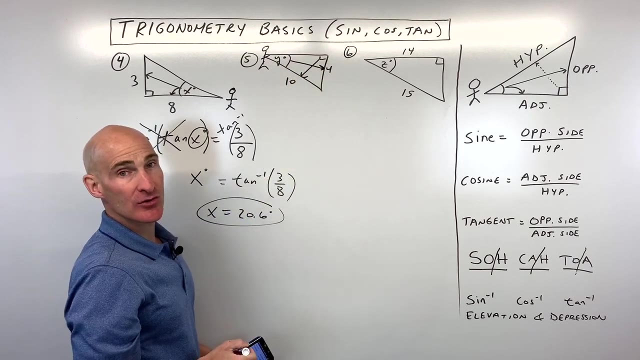 20.6 degrees. So here we solve for the angle. How about for number 5?? Same idea We're trying to solve for angle y. now We position ourselves at the angle and we say what trig ratio ties together opposite and hypotenuse? 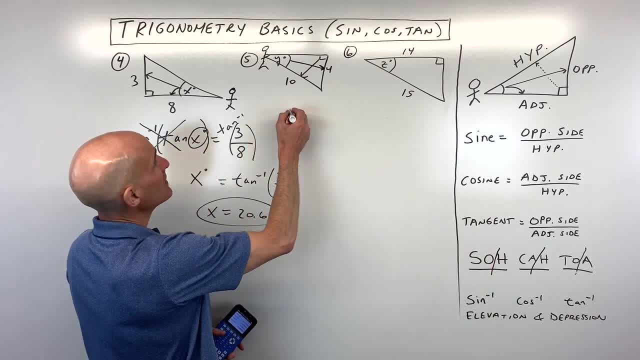 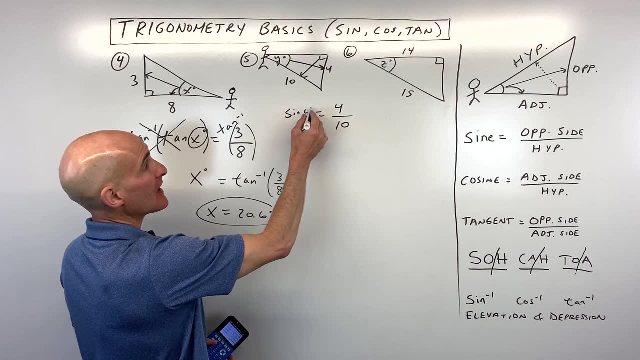 So that one's going to be opposite hypotenuse, That's so, or sine. So we say the sine of angle y equals opposite 4, over hypotenuse, which is 10.. Now again, to get the angle, we're going to go to the calculator. 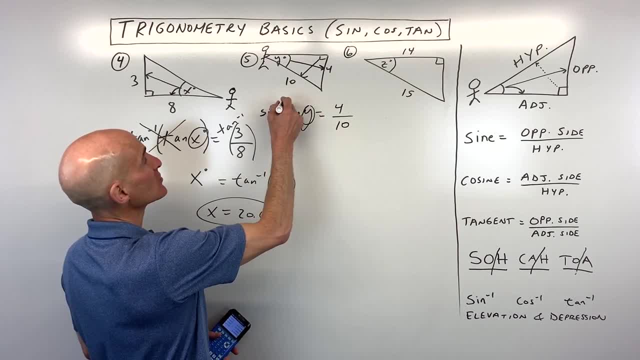 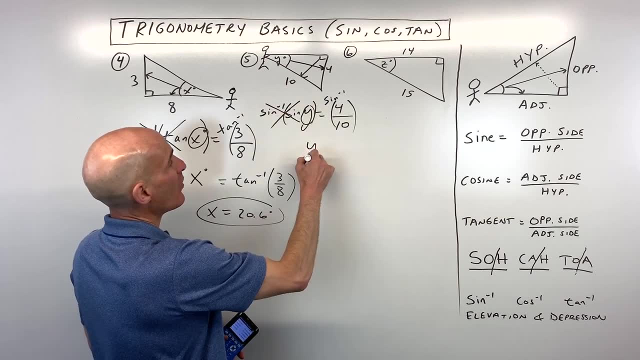 We have to get rid of the sine here. We want to do the inverse. We're going to take the sine inverse of the left side and the sine inverse of the right side. So we get y by itself now And we're going to go to our calculator. 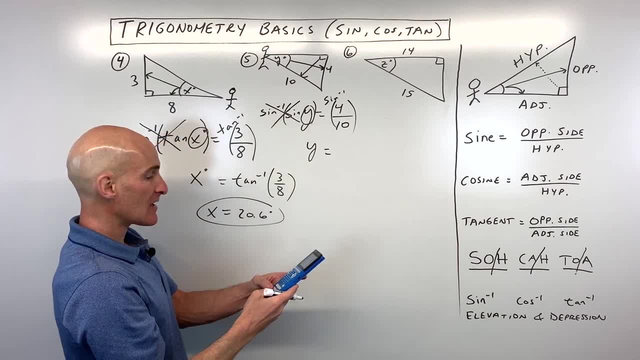 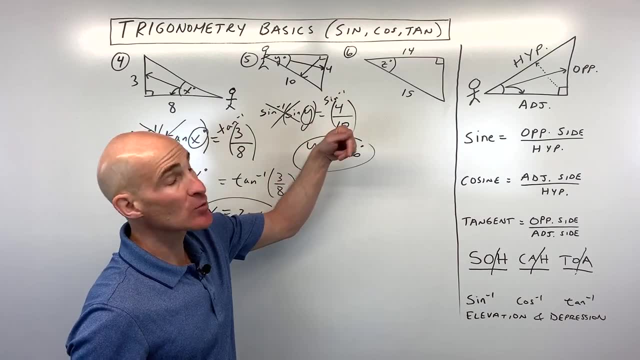 Sine inverse of 4 divided by 10, which comes out to an angle of 23.6 degrees. Last one: See if you can do this on your own And after this we're going to do some problems involving angle of elevation and angle depression. 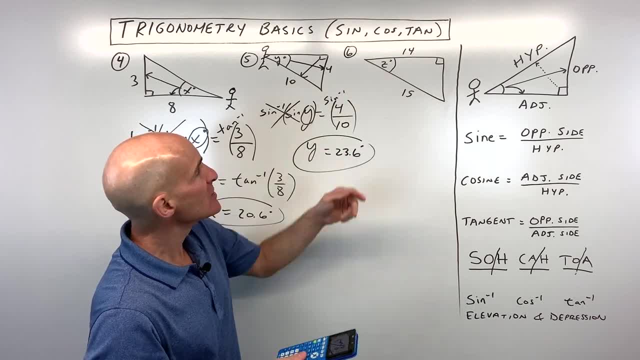 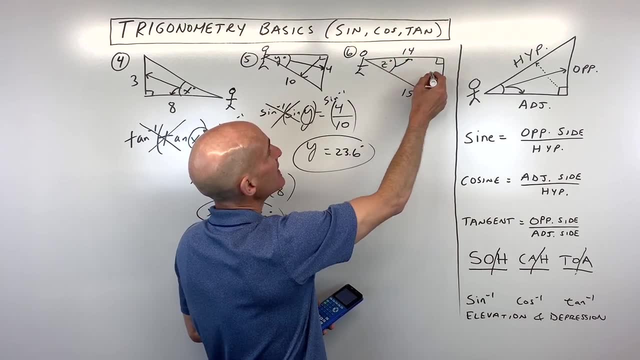 So more like word type problems or stories. So what do you think? Is this one going to be sine cosine or tangent? Well, let's see. We position ourselves at the angle. We've got the adjacent side and the one across the right angle, which is the hypotenuse. 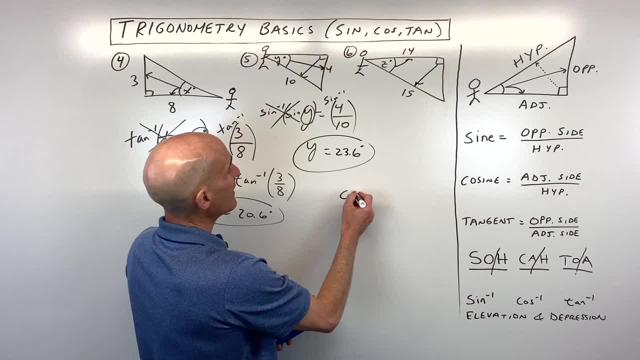 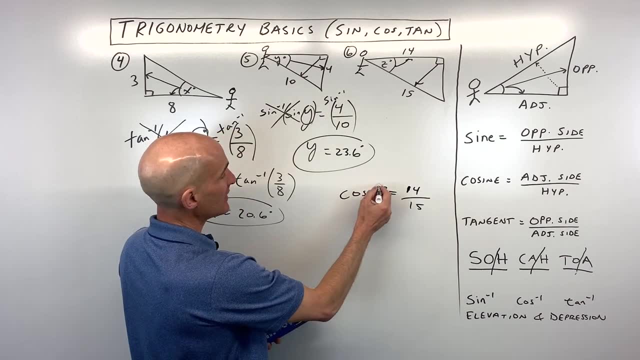 So adjacent and hypotenuse, that's cosine. So we've got cosine of angle z equals, adjacent, which is 14, over hypotenuse, which is 15.. We want to get angle z by itself. So we're going to take the cosine inverse of both sides. 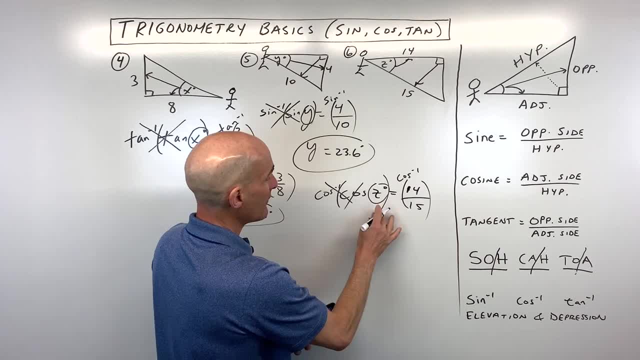 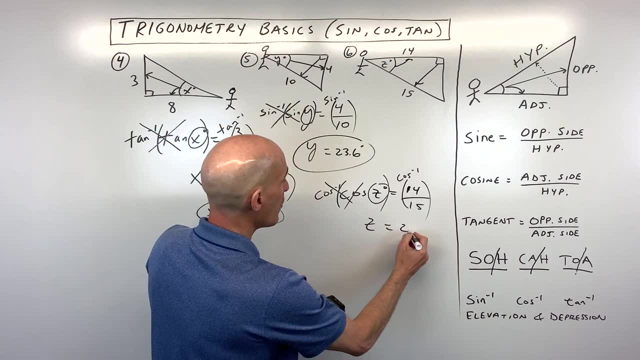 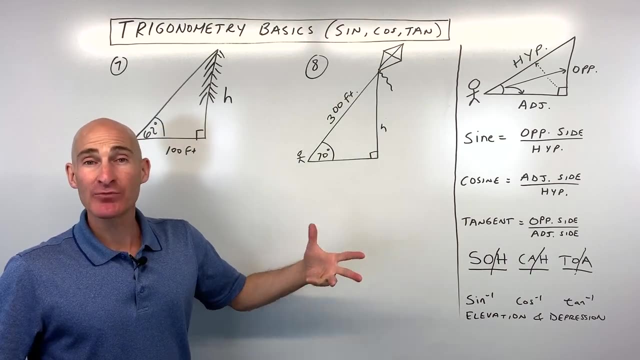 Keep it balanced right. So now we have angle z by itself And, going to the calculator, cosine inverse of 14 over 15. That's 21.0 degrees. is that angle, Before we do number seven and number eight, these application problems with angle of elevation. 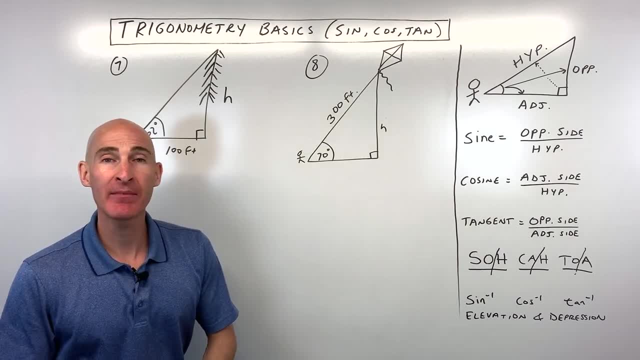 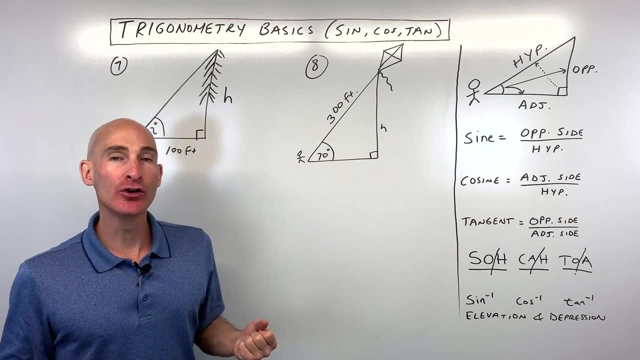 angle of depression if you're new to the channel and we're meeting for the first time. my name is Mario of Mario's Math Tutoring And I'm a full-time math tutor. I work with students every day And what I try to do is take what I've learned working with 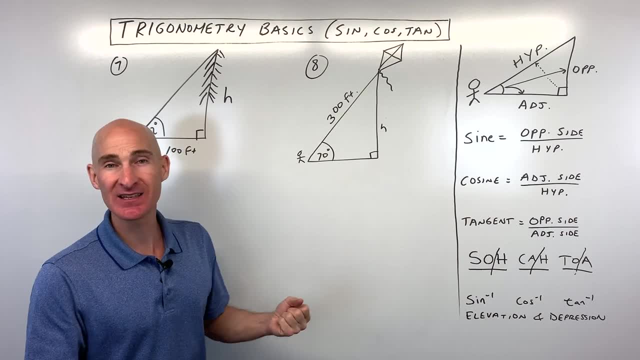 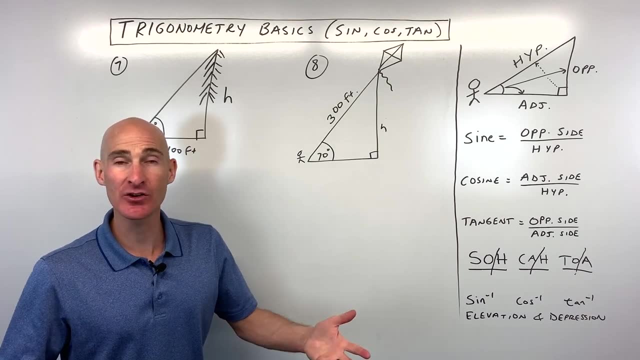 students about what helps them to grasp these concepts the easiest and the quickest, And I incorporate them into these videos so that you can benefit from my math tutoring as well. So if that sounds like something that you're interested in, check out more math videos on my Mario's Math Tutoring YouTube channel. 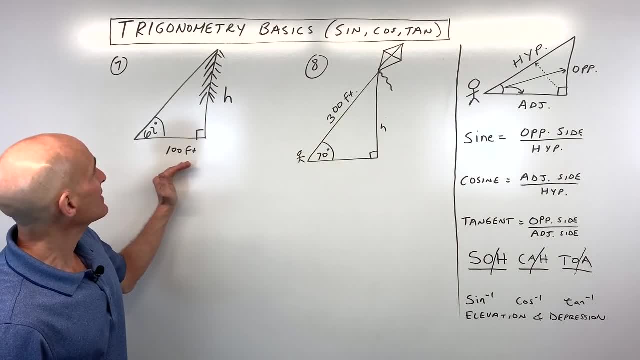 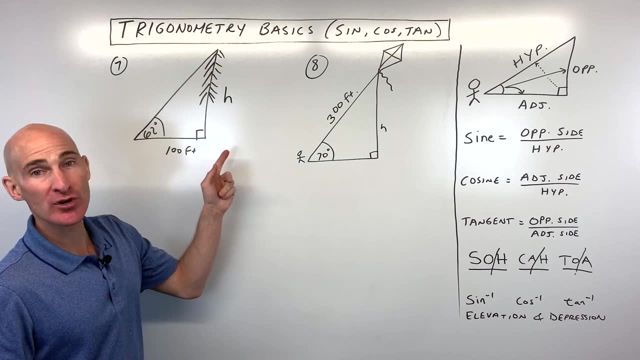 Let's jump into number seven, though. What I did is- I've already taken the liberty of drawing this out for us- just to kind of save space and save time. But say, for example, you're trying to find the height of a tree. 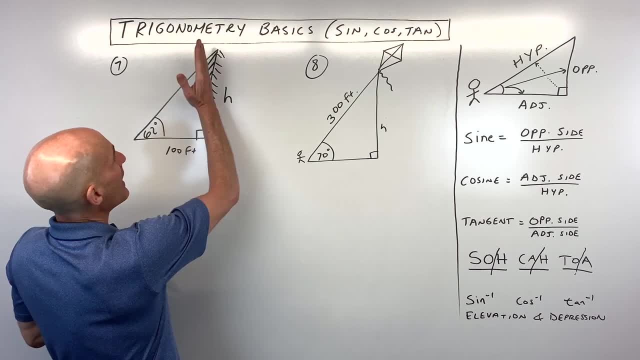 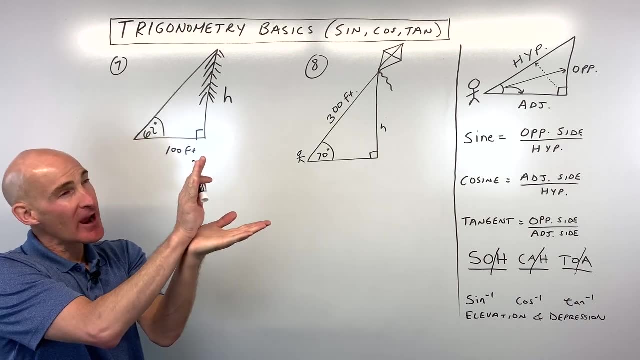 And my drawing's not perfect here. The tree's a little bit crooked. But imagine this tree. It's a vertical straight up and down And you walk back from the base of the tree 100 feet. You get out your protractor. 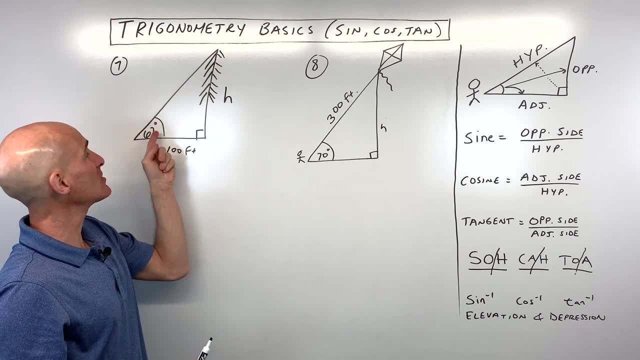 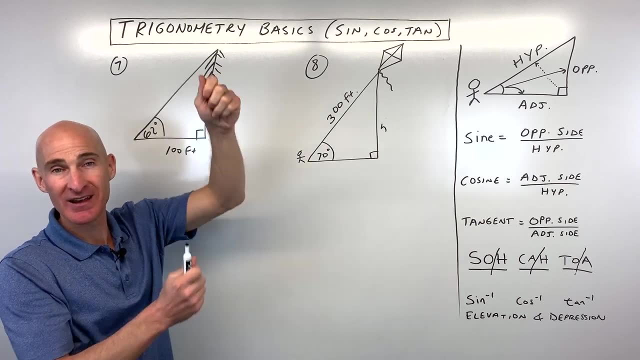 And you say, hey, that angle of elevation to the top of the tree is 62 degrees. How can we figure out how tall that tree is without actually having to climb up the tree and measure it with a measuring tape, right? Well, the first thing I want to talk about, though, is angle of elevation. 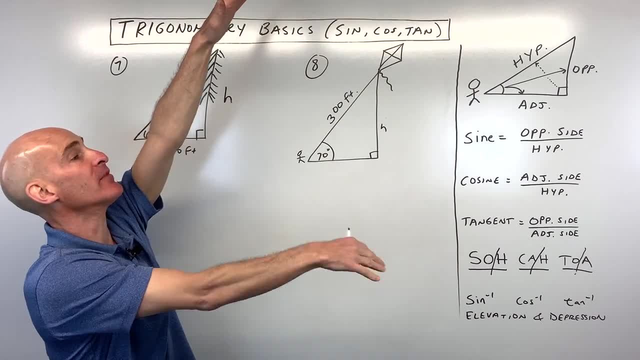 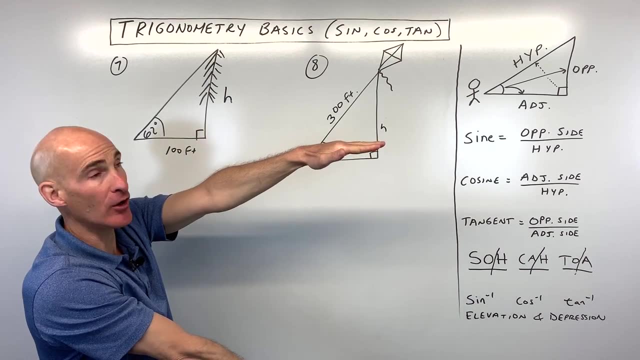 When you think of elevation, it's like you're elevating or you're looking up. That's the angle that we're talking about right there, Whereas angle of depression, you're looking up, You're looking down from the horizontal. OK. 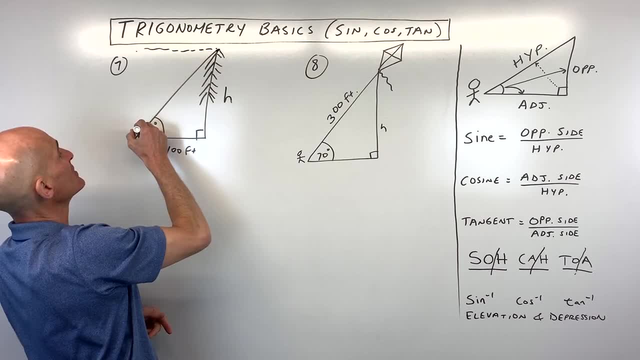 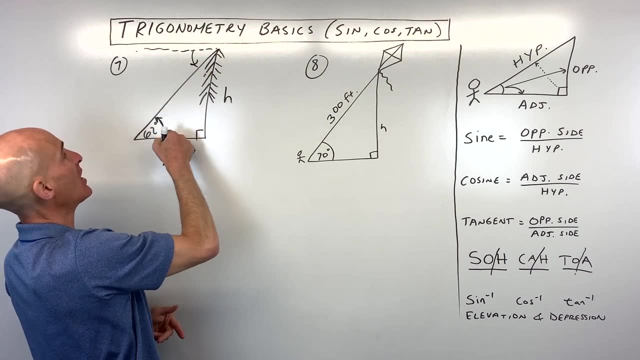 So, for example, if there was a bird up here and the bird was looking down at you, that would be your angle of depression right there, Not this angle, but the one down from the horizontal. This is the angle of elevation up from the horizontal. 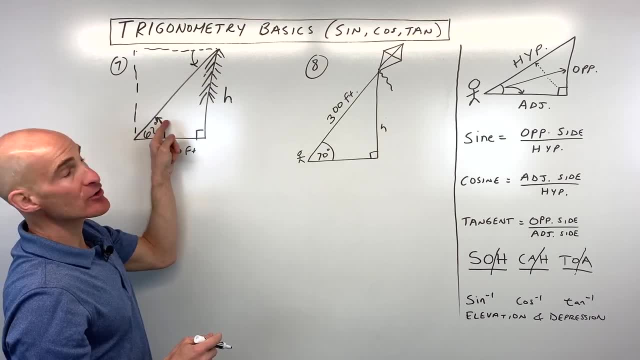 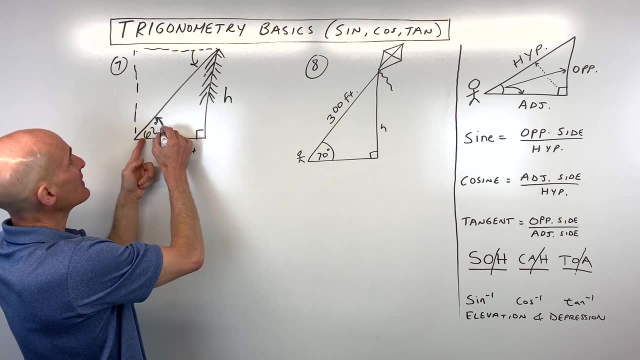 And if you remember from geometry, these are actually alternate interior angles And they're congruent. So if this is 62,, this is 62. So that's something to kind of be aware of. But here we're trying to figure out the height. 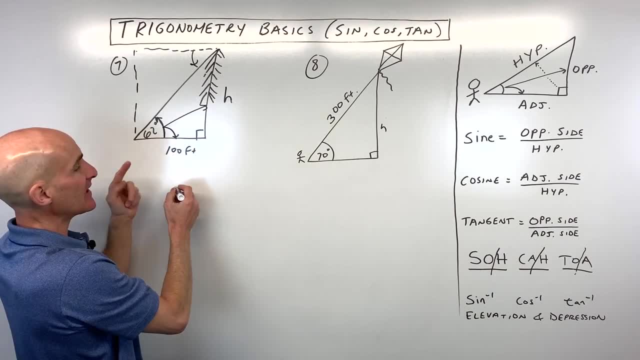 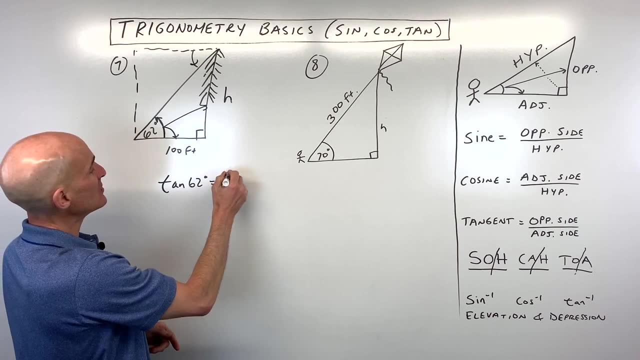 This is the opposite side, This is the adjacent side. So which one's opposite And adjacent, That's TOA or tangent. So we say the tangent of 62 degrees equals H, which is opposite, over adjacent, which is 100.. 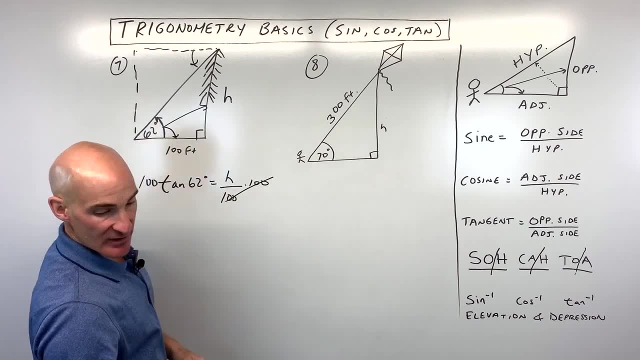 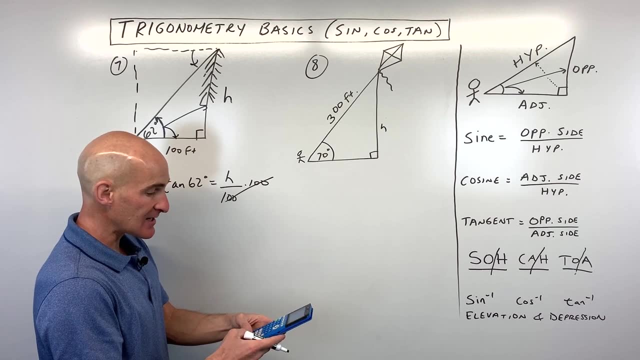 All we have to do now is multiply both sides by 100. And we've got it. Let's see what that comes out, to See how tall this tree is 100 times the tangent of 62 degrees. A lot of times students will say: you know, Mario, you know when are we ever going to use this? 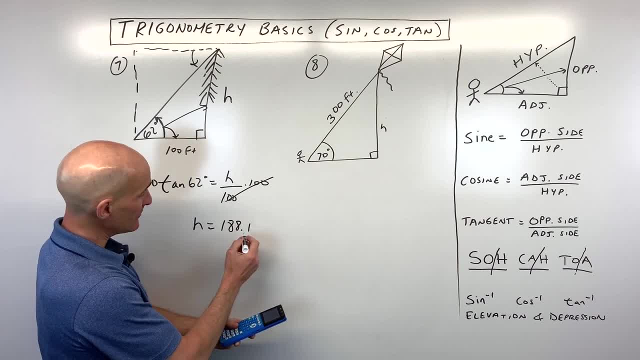 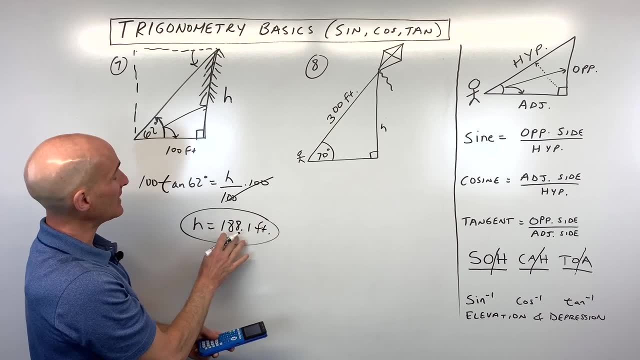 And you know, trigonometry is really very useful. So you can see, We didn't have to climb that tree, We could just stand on the ground and we could get a pretty good estimate of how tall that tree is- 188.1 feet. 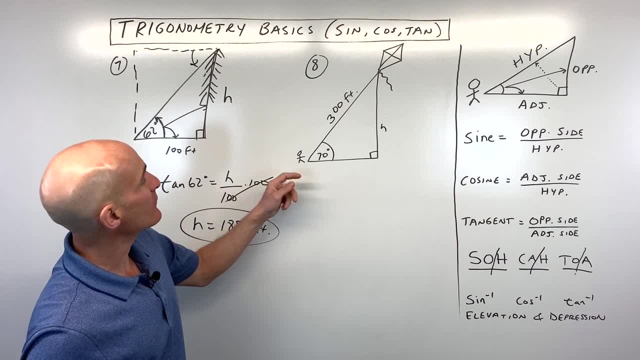 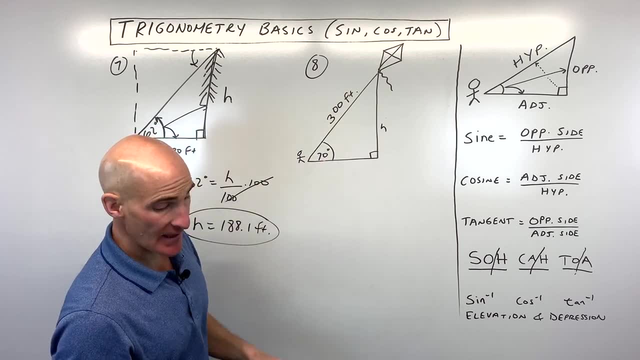 Okay, So let's look at number eight now. This one is a little bit different. We're flying a kite and we let out all the string that we have, And we know it's a 300 foot roll of string. We measure that angle of elevation right up from the horizontal. 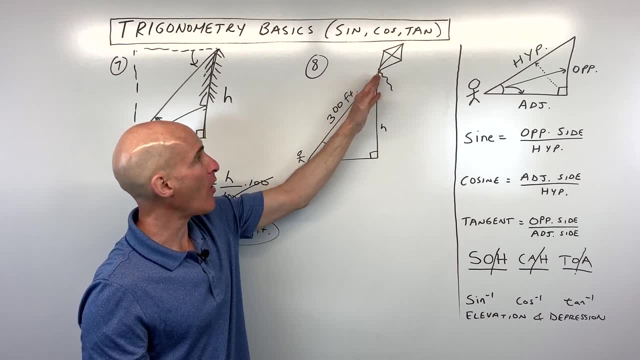 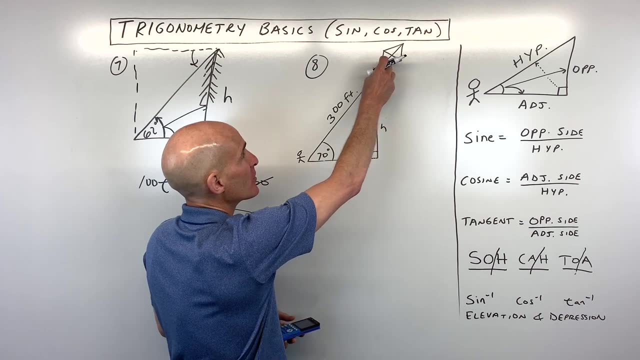 We say that's a 70 degree angle, Okay, But we want to know how high is the kite actually above the ground straight down? Okay, Well, of course we can't, You know, jump up here and put a measuring tape and measure that. 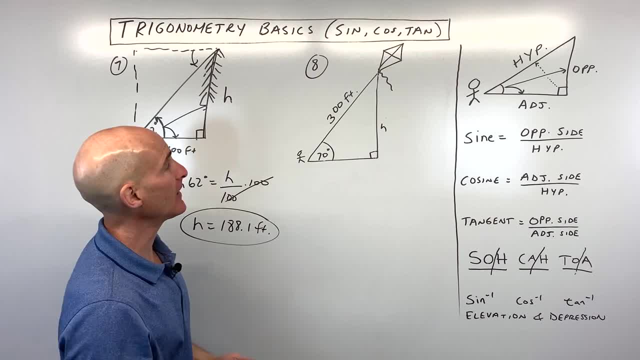 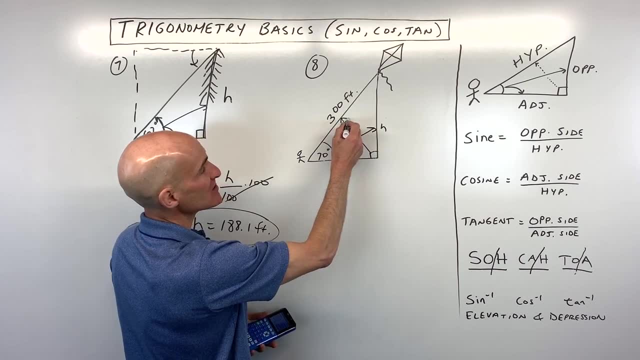 Right. So here's where we're using our triangles, our trigonometry, Right? So what trig function do you think ties together this angle, this side which is opposite, this side which is hypotenuse? Hmm, Opposite and hypotenuse. 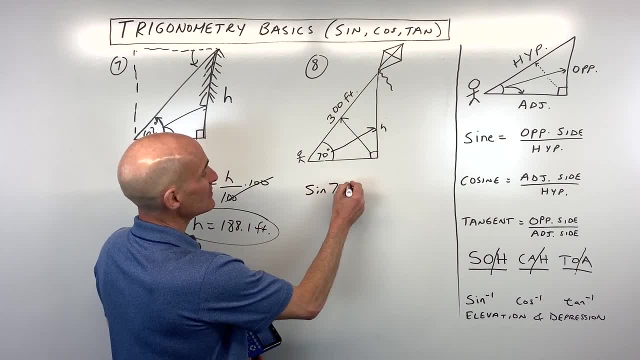 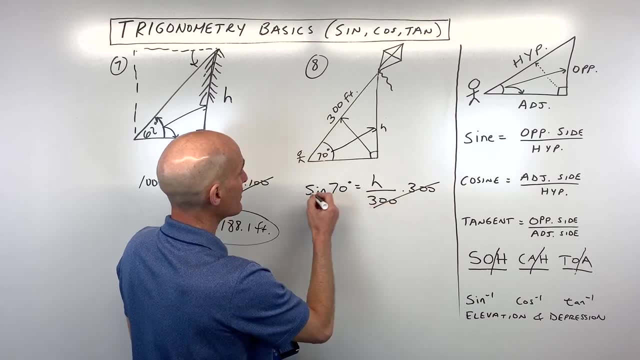 That's so, or sine. So we're going to say: the sine of 70 degrees equals the opposite, which is h over the hypotenuse, which is 300.. Now all we have to do is multiply both sides by 300 to keep it balanced. 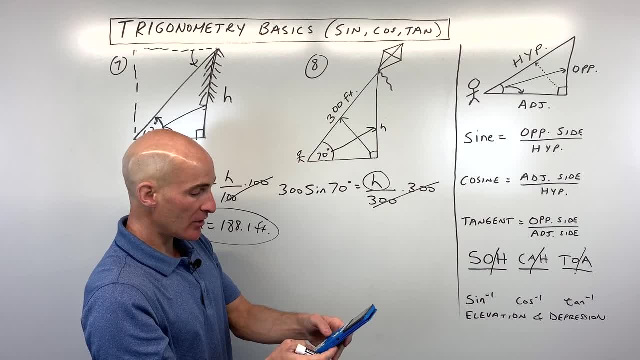 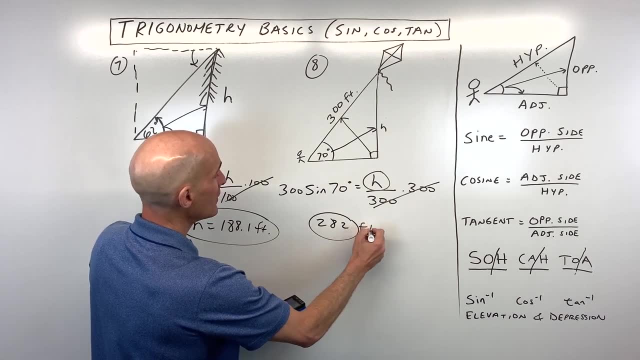 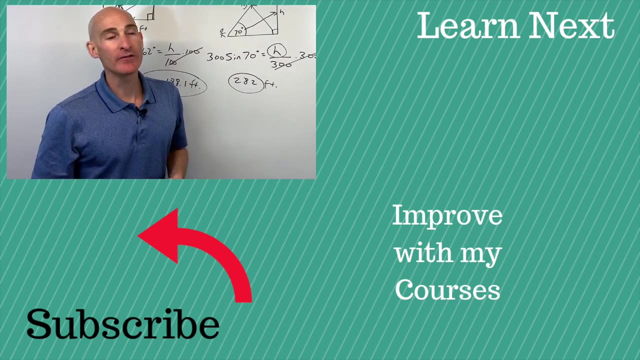 Get that h by itself And go to our calculator. 300 sine of 70 degrees is 280.. I'm just going to round About 282 feet above the ground. If you like my teaching style and you want to learn more about trigonometry, follow me. 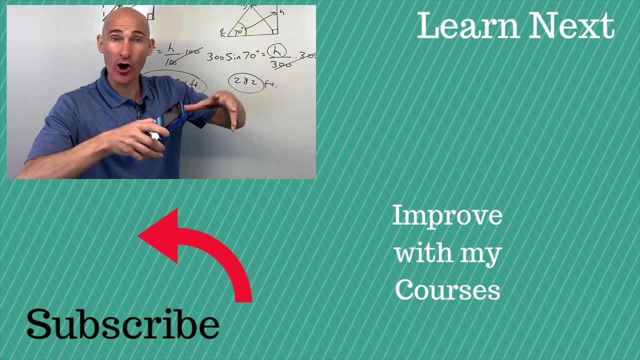 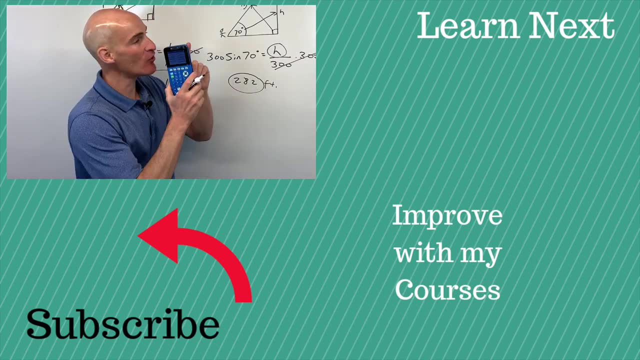 over to that video right there where we dive into how to solve right triangles, meaning you're finding all the angles, all the sides. It's usually the next step when you're learning about trigonometry. So I'll see you over in that video.